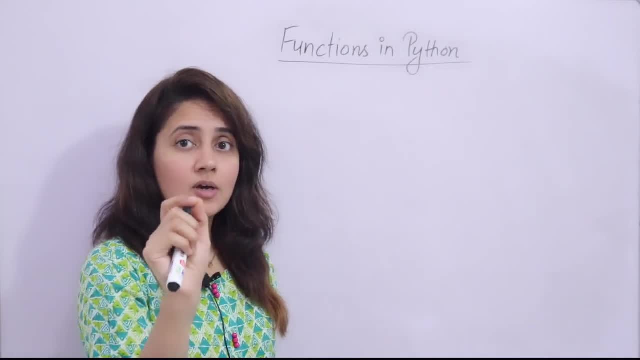 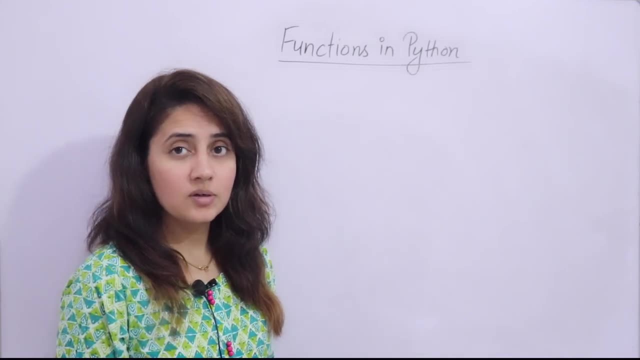 about function. what is a function? why, basically, we need a function? this answer, this question, is very important. why functions? what are the benefits of using function? how to define a function, what are different types of function? right, with the help of real life example, I'll tell you what is. 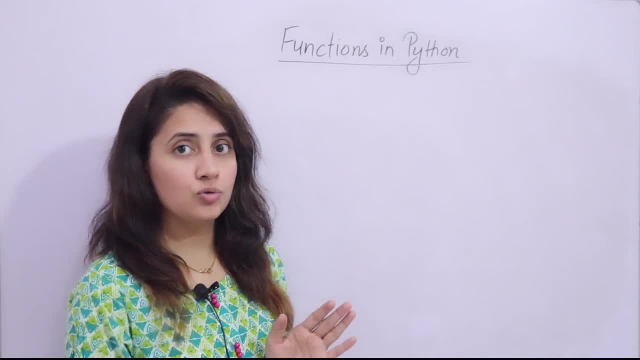 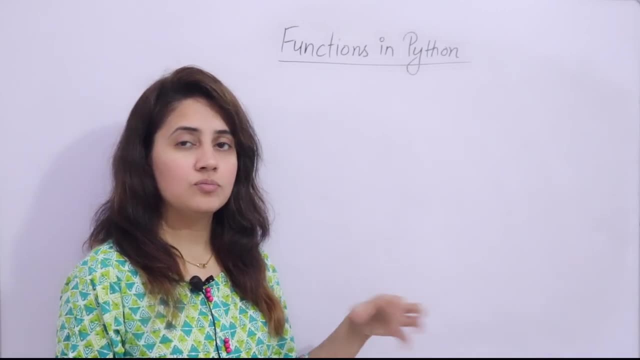 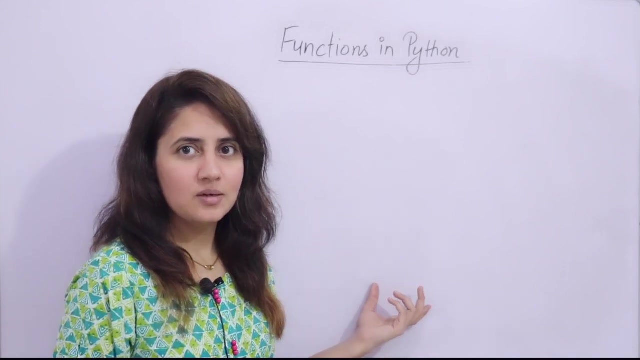 function and, with the help of program, also practical. also. I'll show you and I will introduce you with a new tool, also in this video. after using that tool, you will be- you know, you know- very friendly. you can say with functions, right, it would be very easy for you guys, maybe someone of. 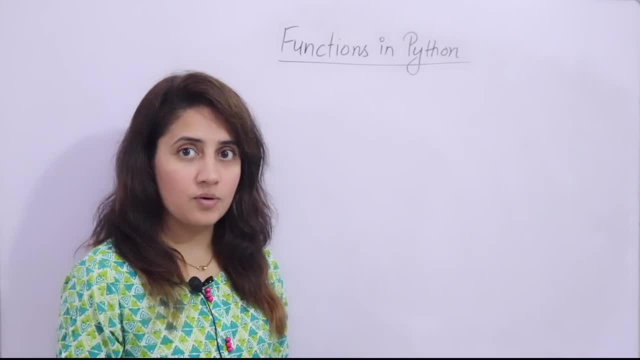 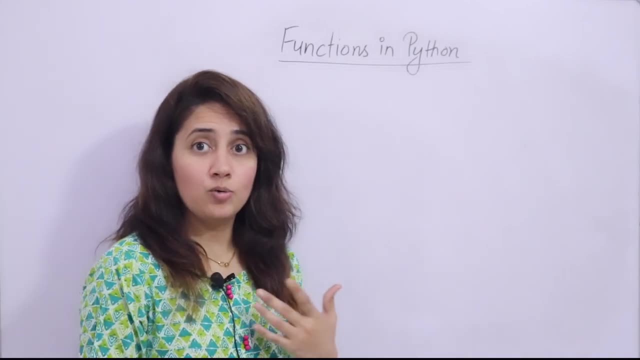 you are aware about functions. they have learned other languages- cc plus for java. but let's start this with a real life example. suppose I know I know a recipe, I know how to make it idli, one of my favorite from south indian food actually. and suppose one sunday my friend came. 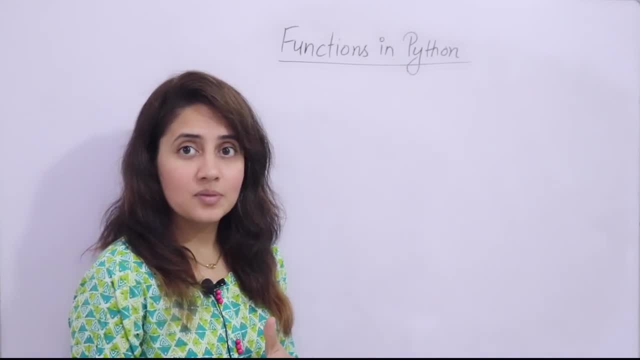 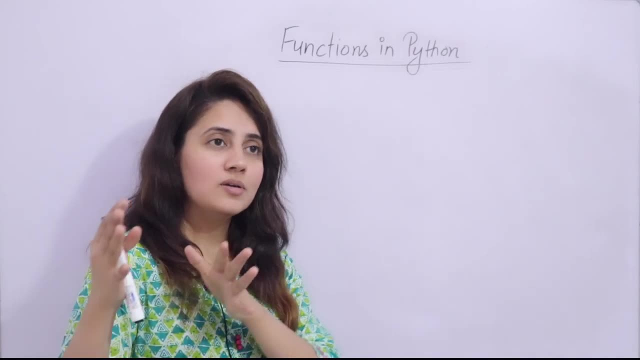 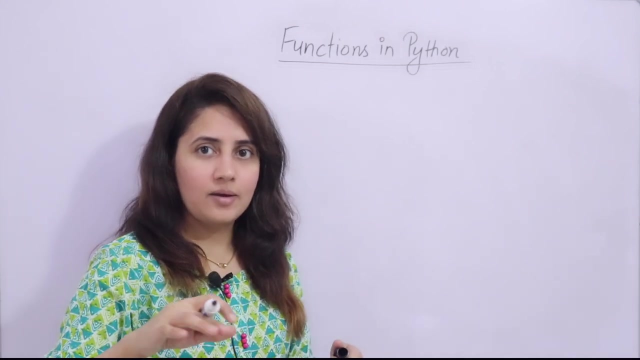 to me came to visit me and I made idli for them and she was like, oh wow, idli, like they, they are so delicious and amazing. so she asked me the recipe for that idli and I told her, like, like this. even to be very frank, I don't know what is the recipe, but let's take, let's assume I know. 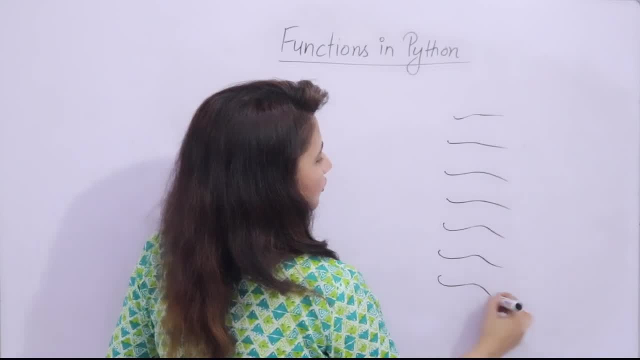 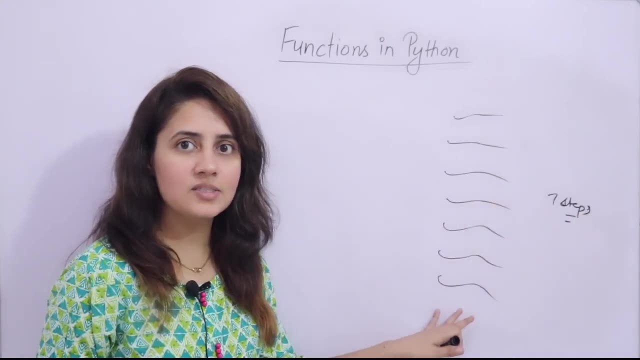 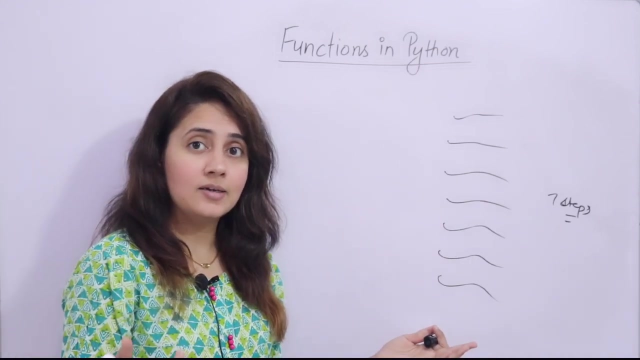 so it was. there are these five or six or seven steps- one, two, three, four, five, six, seven steps in the recipe. so I told her: these seven steps, right? maybe on next day or on another friend came to me and she also asked me for the same recipe because I'm in Italy again. 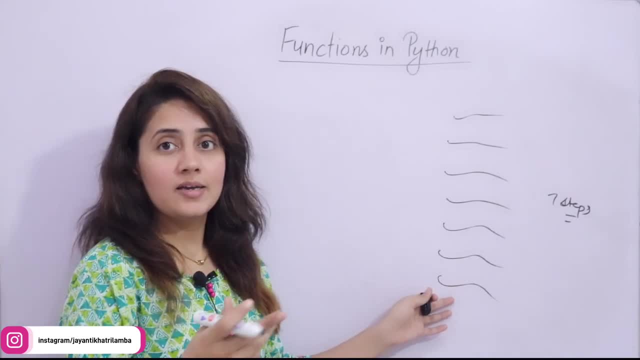 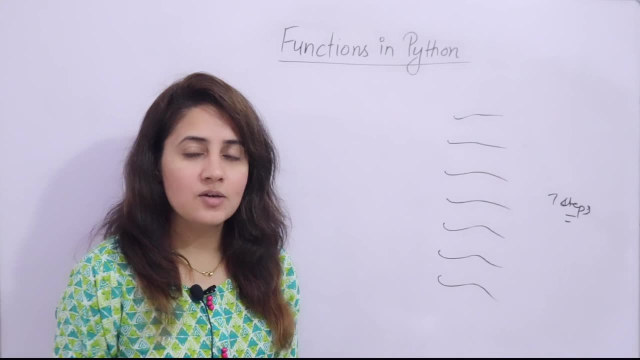 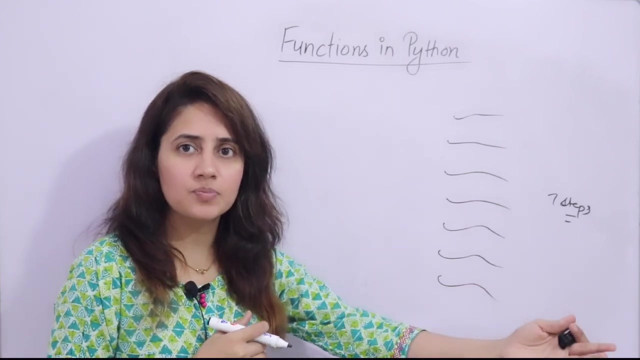 because in this I am export, you can say so. I told her the same recipe like this: maybe every Sunday or every after two to three days, someone is coming to me and I am telling them the recipe. I am repeating these seven steps again and again. I am telling them the recipe, right. 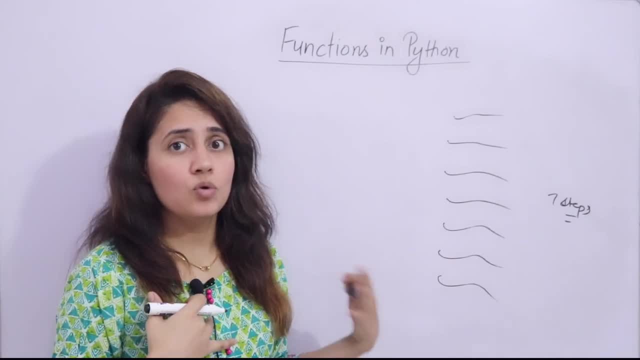 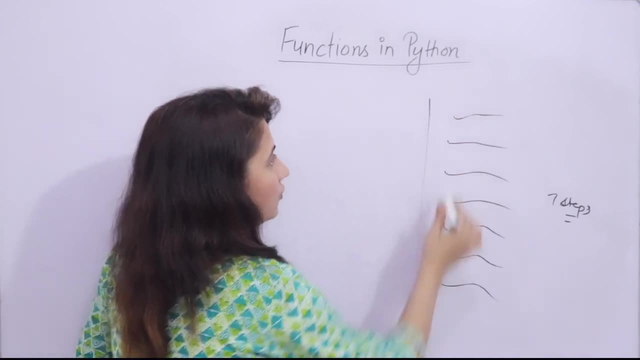 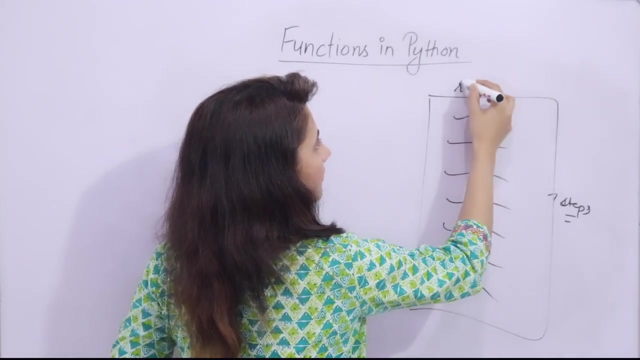 so what I can do, rather than this, what I can do. now I am feeling very frustrated after telling the recipe again, again, again. so what I can do, I can just write down this recipe on a paper right, and like RECIPE recipe of idli you can say making idli right. and whenever anyone comes to me and 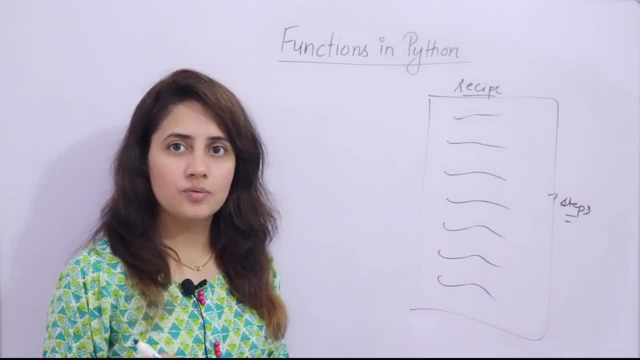 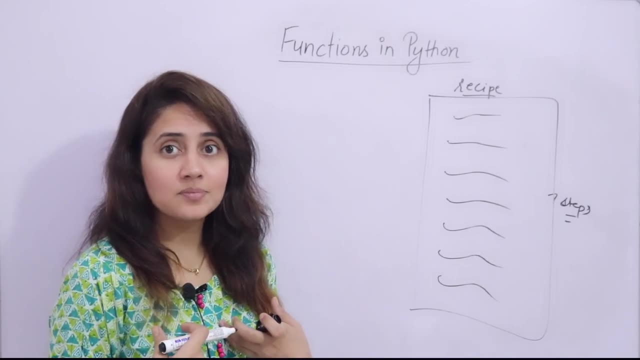 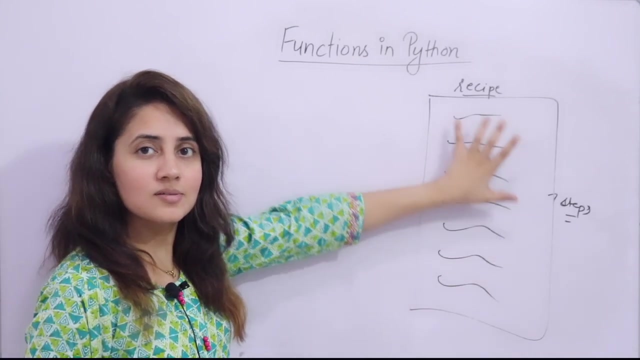 ask for the recipe. I just hand over this piece of paper to them, right? so, yeah, it is going to say what? what is the benefit? my energy and my time, right? I have just grouped these steps in us so you can say an and and this is an entity. this is an entity on a paper, and I will just hand over that paper to 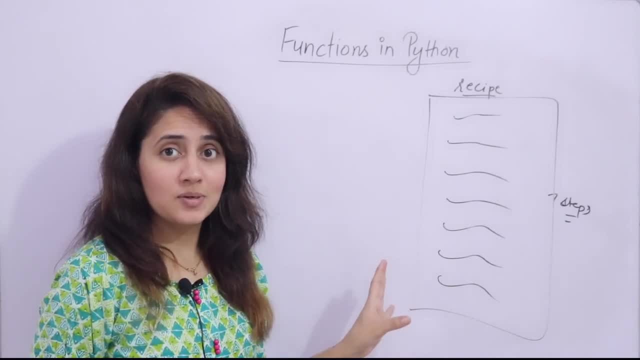 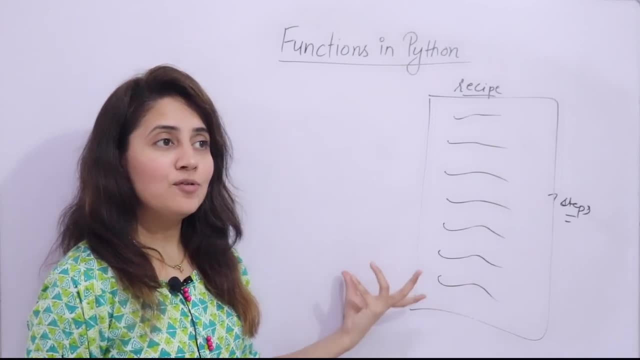 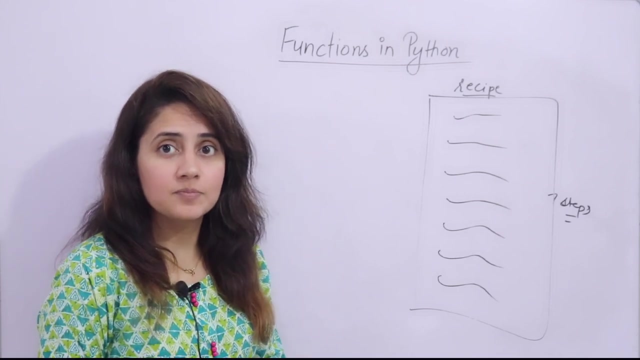 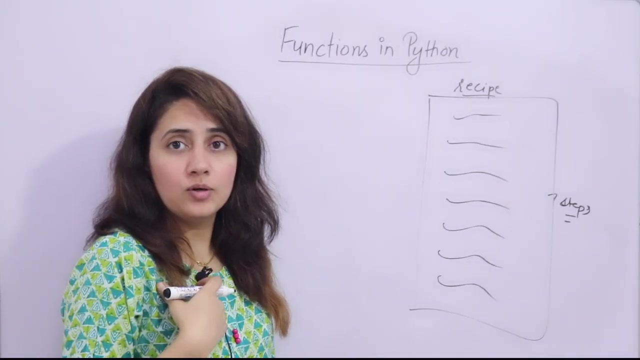 whoever is going to ask me the recipe about the recipe, right? so yeah, this is beneficial for me, right same. we have some function, like in programming. also, we have to do something like some task again and again, right, suppose? let us take one example and see if you take one more example. like we human being also we are performing different. 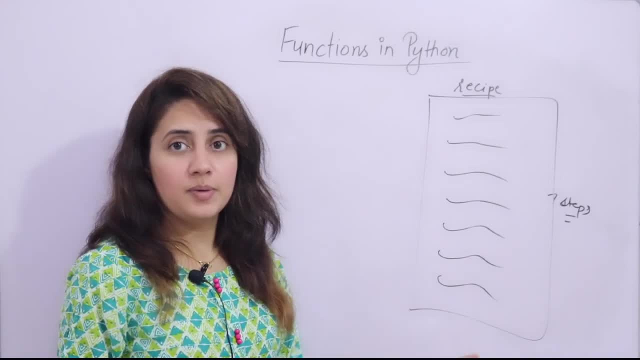 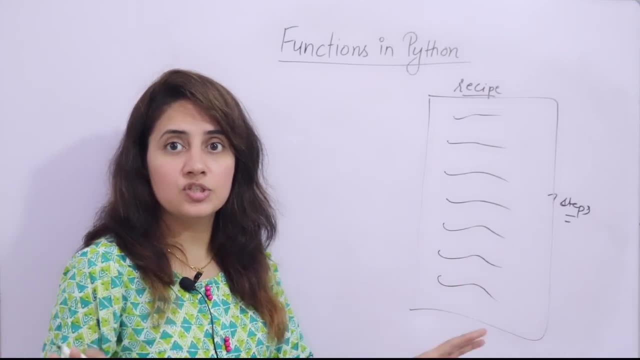 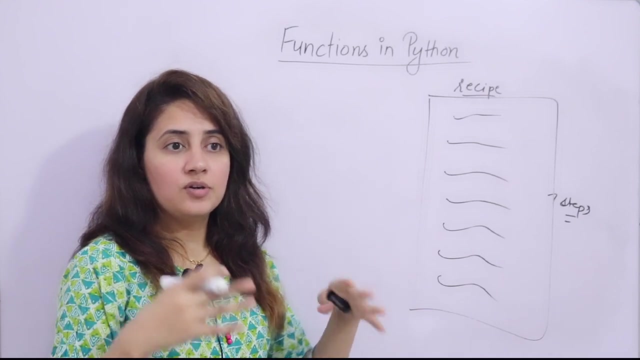 different functionality. we are multitasker, like let us take a female as a mother, as a wife, as a daughter, as a working women, and many functionalities are there right. so different, different functionalities are there for the same entity, for the same person. right means like if you are in front of your 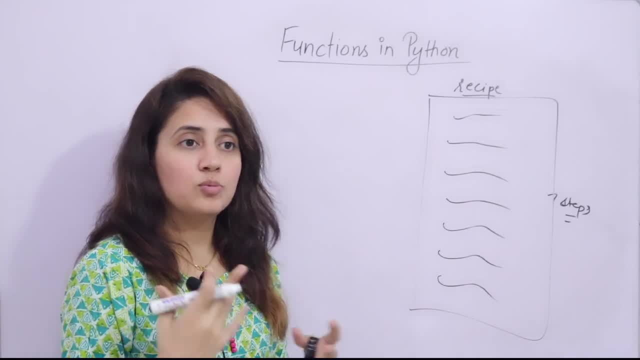 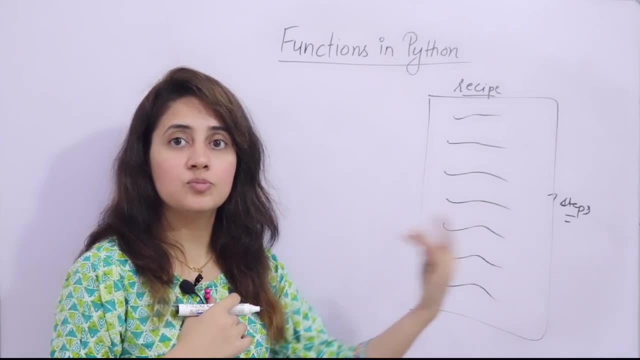 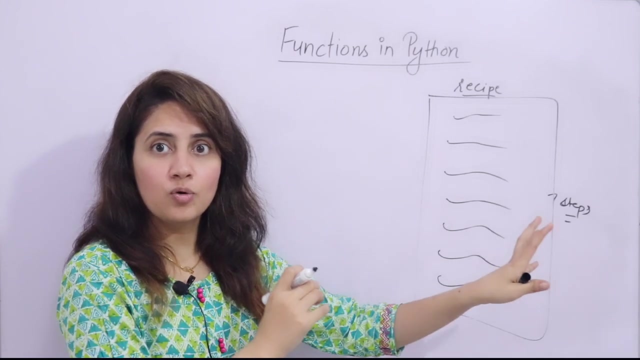 student. you are working, you are, you know. you know your responsibilities work, you know acting as a teacher, right? if you are in front of your children, then your responsibility means your functionality is your working as a mother, something like this: so whatever is in front of you. according to that, 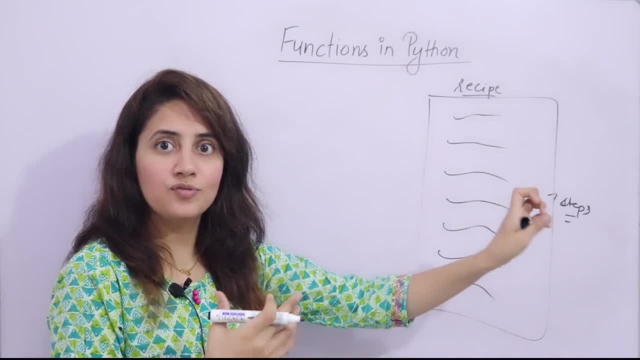 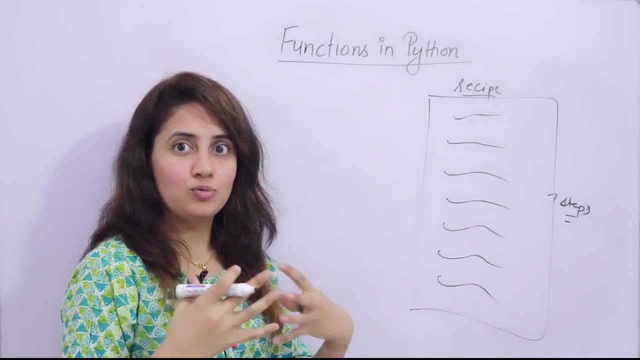 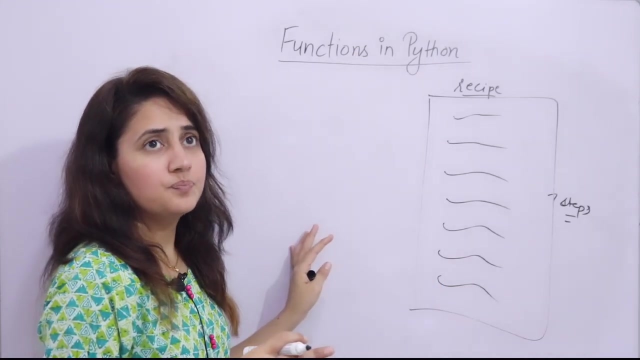 you have to perform your task right for different, different inputs. you are performing your specific task right. so like this example also you can relate with functions. let us take this example: if in programming also like two lines there are two lines, simplest example I am taking, like print. 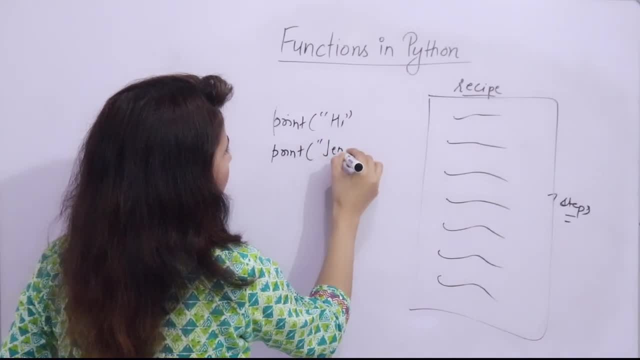 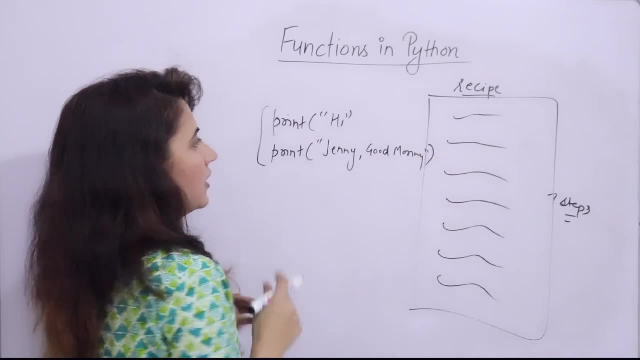 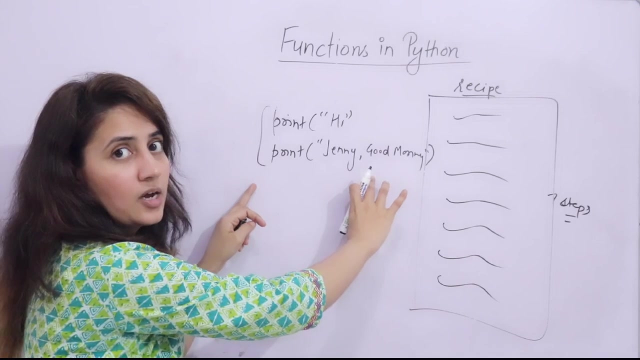 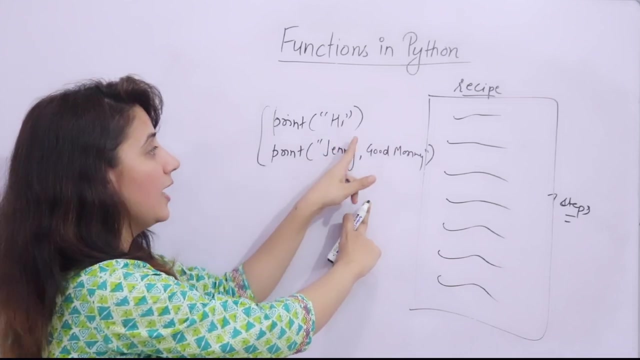 hi and like Jenny, and good morning. like this: I want to print these two lines again and again in my program like: perform some specific task, then execute these line, then perform some specific tasks. then again I want to perform, I want to. you know, greet, like I want to print: hi, Jenny. 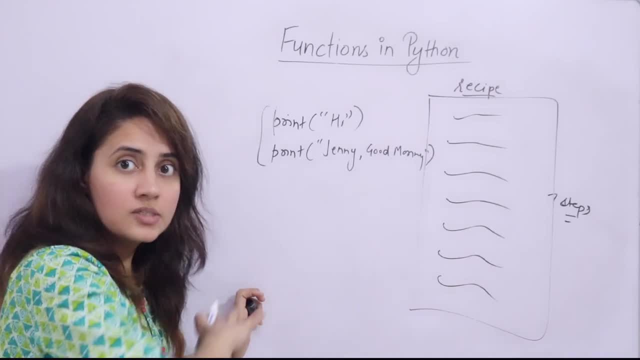 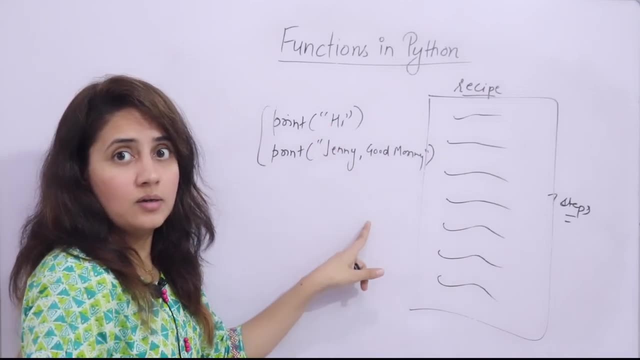 good morning. then again perform some specific task in the same program again. I want to perform these two lines. perform some specific task again. I want to greet like: hi, Jenny, good morning. right in program, maybe 50 times. so 50 times you need to write down these two lines. so, rather than this, what? 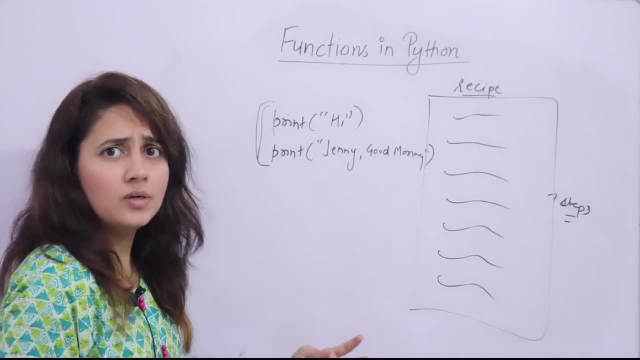 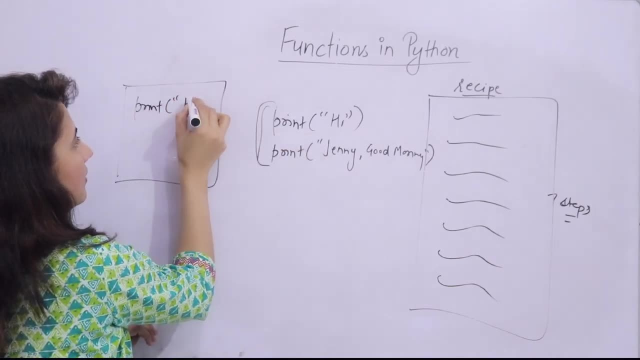 we can do, rather than repeating the two lines again, again what we can do the same thing. just wrap up this thing here like: print these two lines. print then Jenny and good morning. these two lines are all right. so it will say that I want to greet you today, right? so next a user will comment that. young, are you healthy? okay, say hi, Jenny. good morning, J meets you. okay, Los Angeles. this is my website search engine. her name is Johnny Tim Smith and a sister is the child. okay, a student normative like that. so in different code she will say: how are you? how are you but say: powerless here for all other? 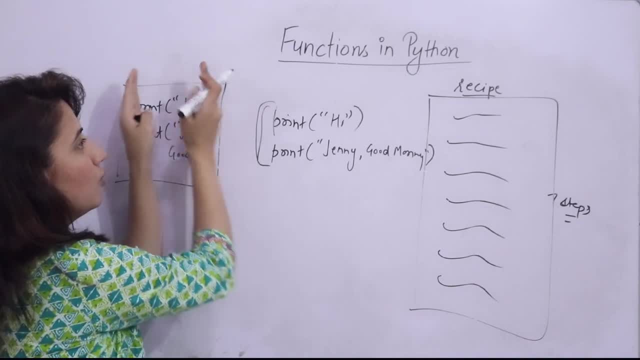 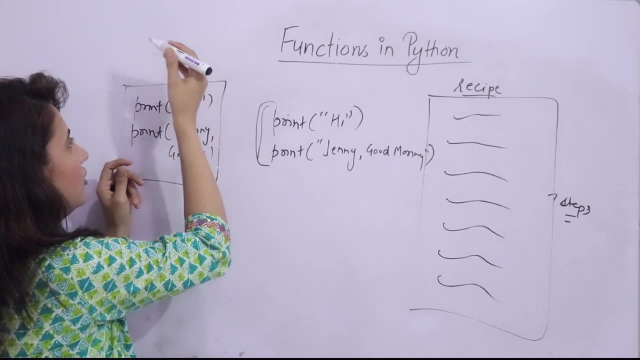 the students. so there is a particular agreement up there. students writing thatですね will come up lines here, right, And just call it what I am calling this: a recipe, right? So it's like you will say a function name, So let's call this thing. what A function name: greet And. 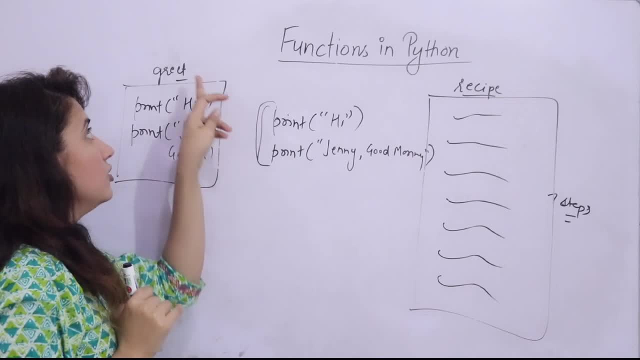 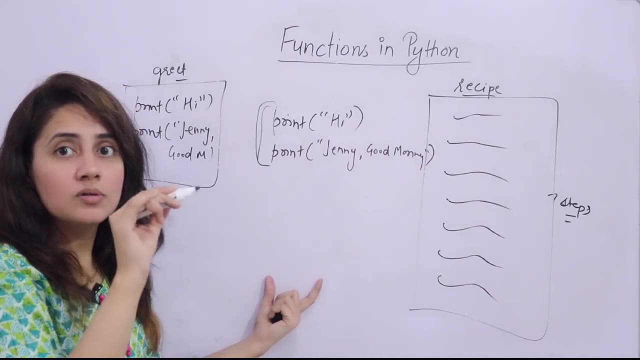 whenever you want to execute these two lines, then just call this function: greet, greet, greet. So rather than writing these two lines again and again, just have to write down simple function: name: greet. that's it, right Now I will tell you how to define a function. 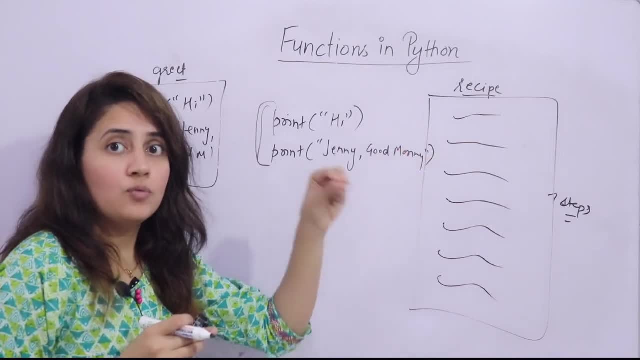 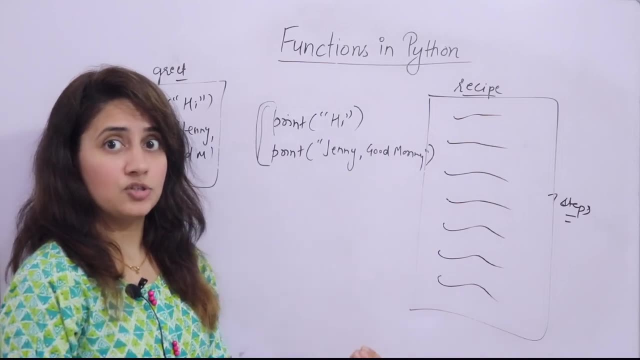 how to call the function. There are two major steps, basically. First of all, you have to define a function, then you have to call the function right. So now I hope you got it. What is basically a function? Function is just what: A block of statements or a block of code. This is just a. 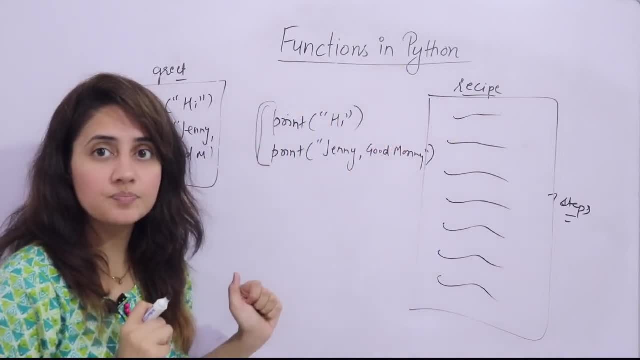 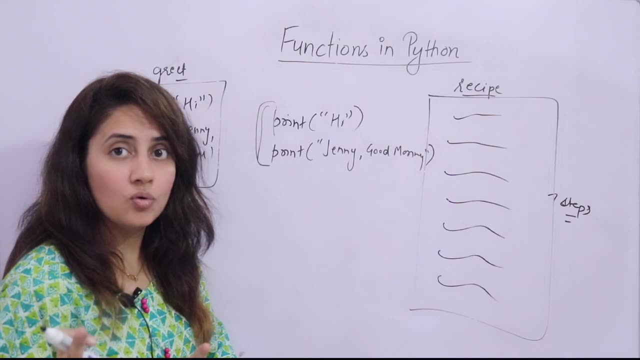 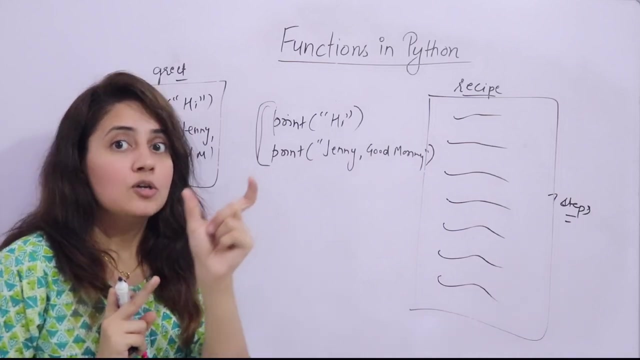 block of code. This is just a block of code or statement. These are statements, right, Which perform some specific function. When it is called, it is going to perform those tasks. only when you are going to call that function. These lines are very important. So when it is called so, function is a group. 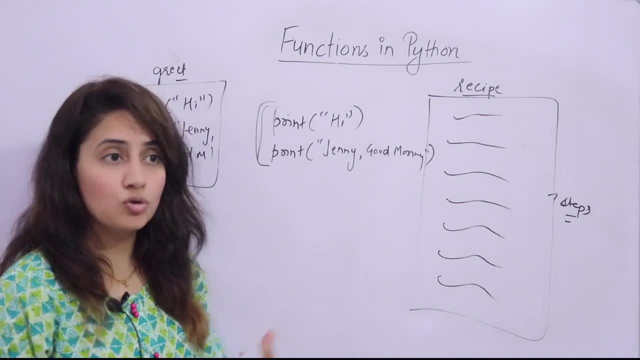 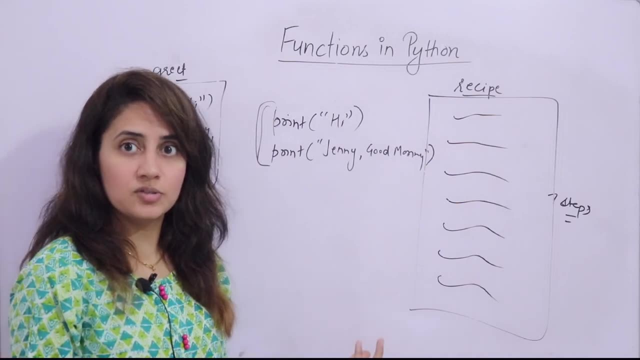 of you can say it's a block of statements or block of code which is going to perform a specific task, which perform a specific task when it is called. That is function definition. Very simple right Now, how to define a function. Let me tell you. 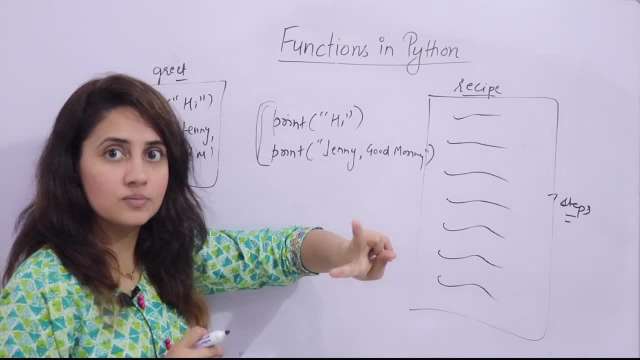 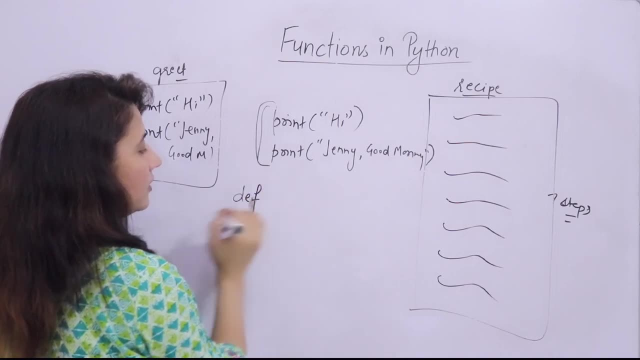 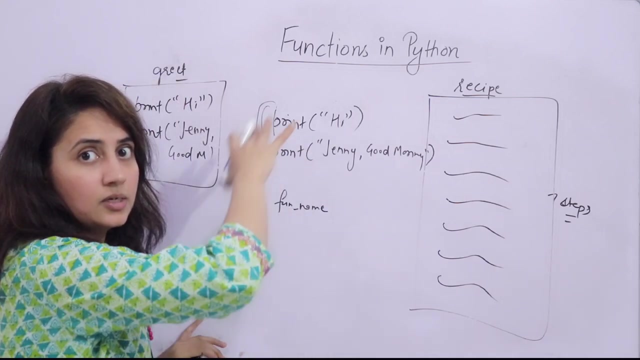 Two steps I have told you. First, define a function, then call the function right. So how to define a function? Simple. What is the syntax? You will write down this def, keyword, d, e, f. Then here you will write down your function name, any name you can take, like add, subtract, greet- any function. 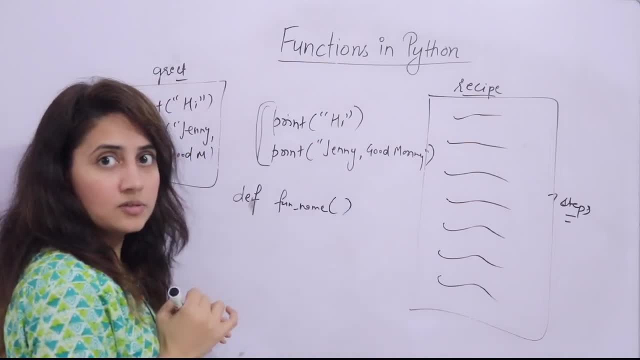 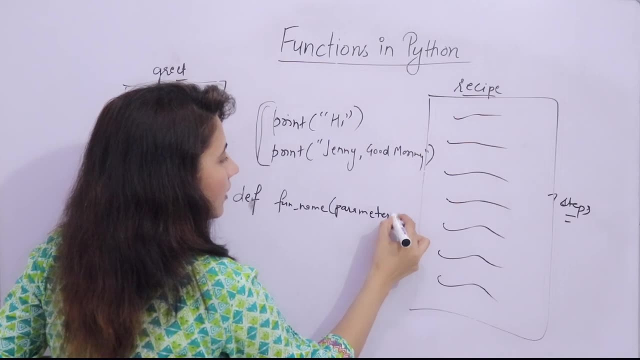 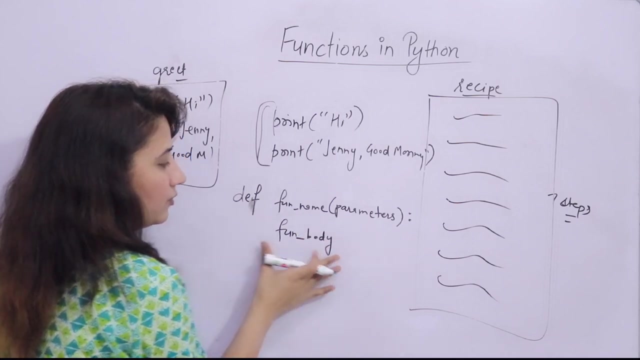 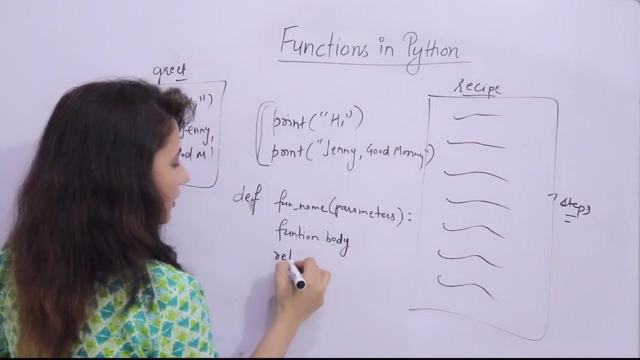 name display anything. These parenthesis, then colon, or in these parenthesis, if you want to pass, you can pass Parameters right. Then here we have, here we have function body. or let me just write down this thing: Here we have function body And after that we have like return, return. 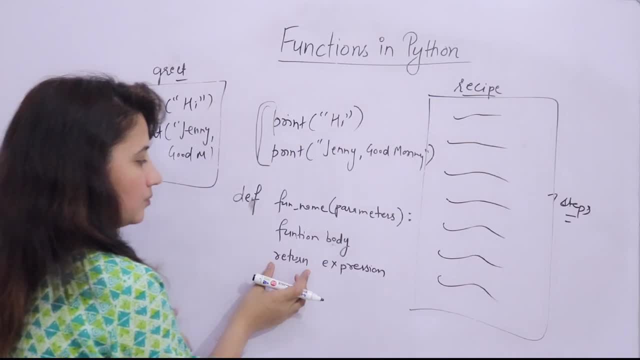 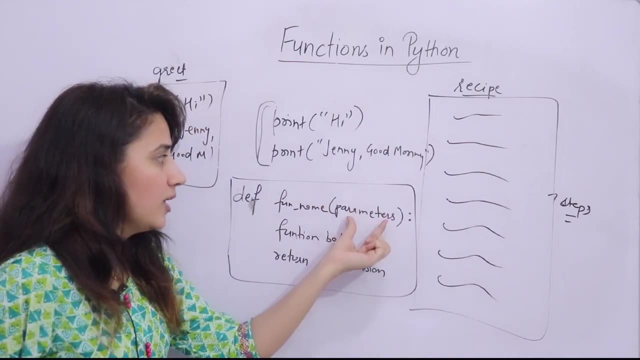 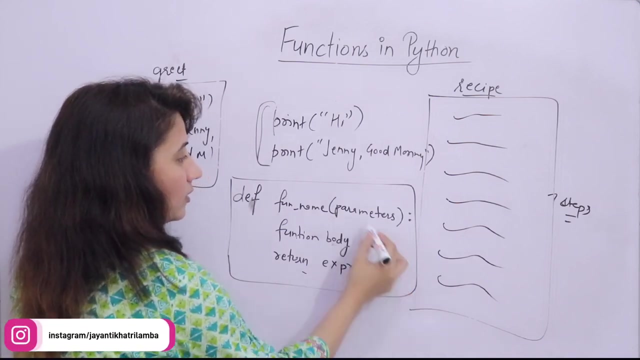 statement, Return keyword, and then some expression or whatever you want to return. So this is what, the complete one. It is not necessary to pass parameter every time. It is not necessary that every function is going to return To return something. So this line is optional, This one, these parameters are optional, But 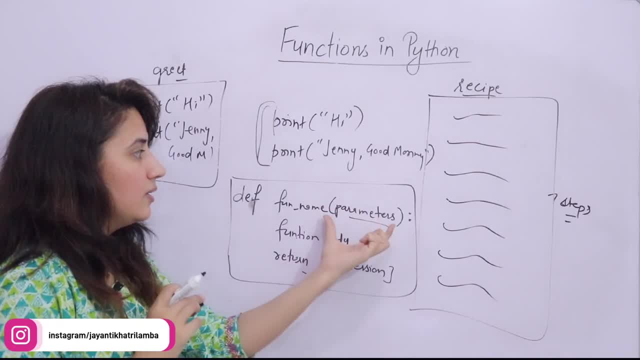 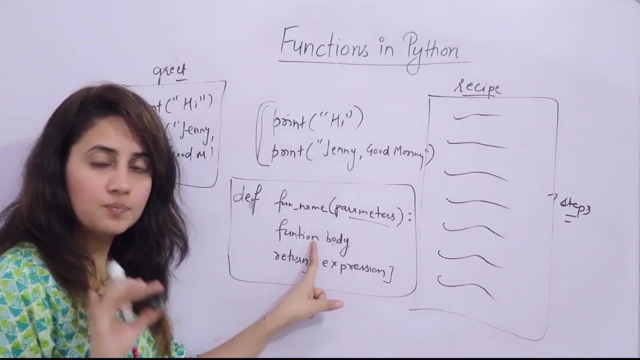 the mandatory part is to define a function def, keyword, function name, these parenthesis, maybe these are- empty this colon and then function body: right. These are important. These are, you can say, mandatory part if you are going to define a function Parameters. 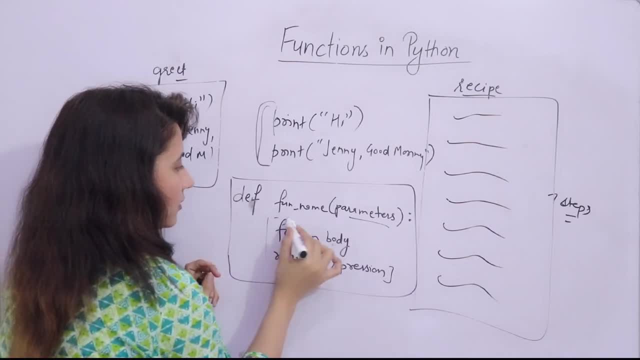 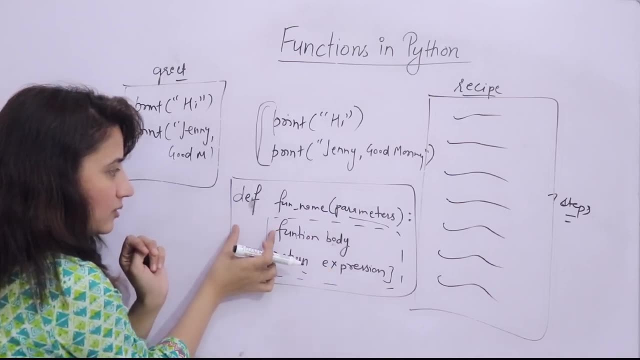 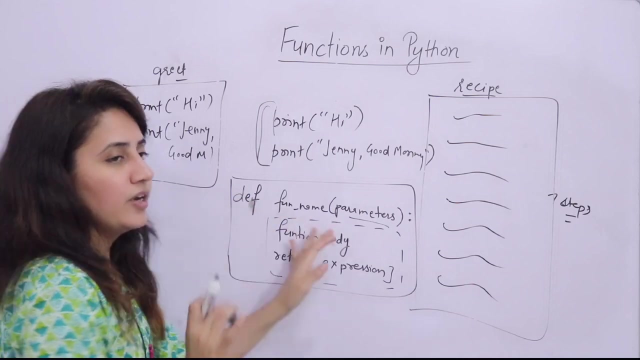 return expression. these are optional part right. And this: this: this should be indented Right. See, I have. there are some space at the beginning of these two lines, So these should be indented, Otherwise it will give error, Right? So this is. you are going to define a function. How? 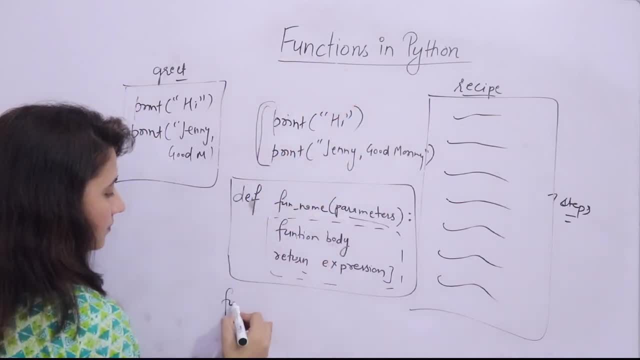 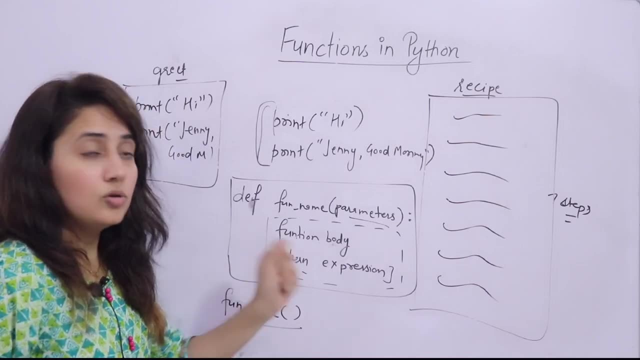 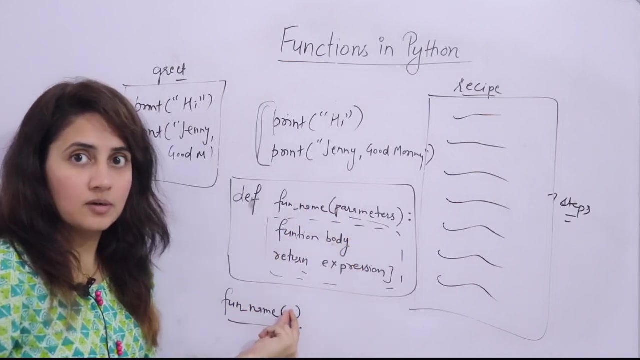 to call the function, then Just write down the function name- Whatever the function name, and these parenthesis: If. if you have passed some parameter, if you have used some parameter when you are defining a function, then you have to pass those parameters here: 1,, 2,. 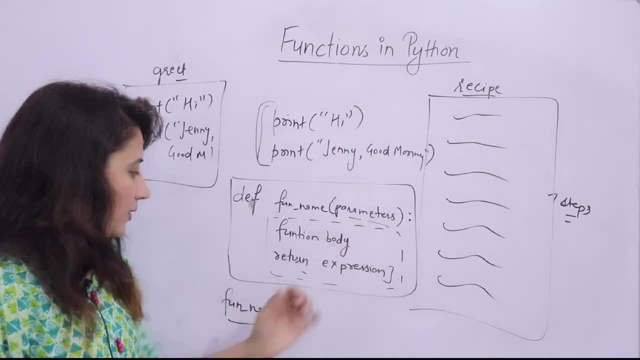 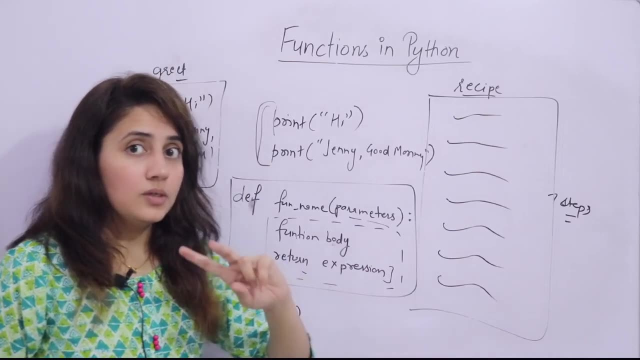 3 or how many? 4.. How many parameters you have? If there are no parameters, just function name and these parenthesis. This is what you are going to call the function Right Now, and function will only work when you are going to call that function Only. definition of this function. 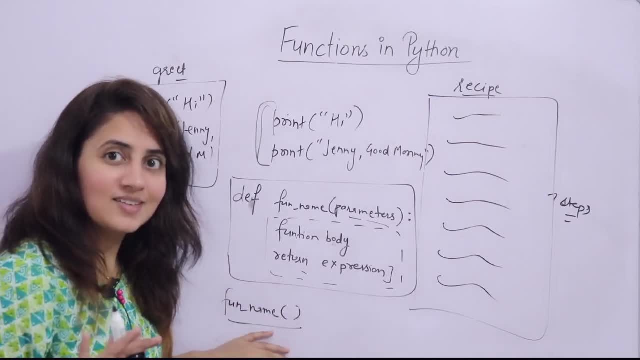 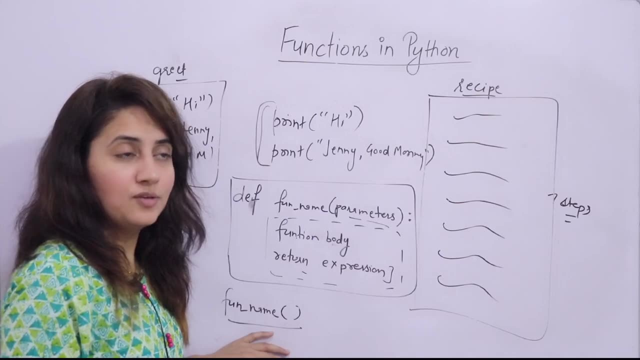 this is not going to work. You have to call that function Right. Like me as a teacher. So whenever I am in front of my student, right In front of my class, then only I will act as a teacher, Right? So whenever I am in front of my class, then only I will act as a teacher. 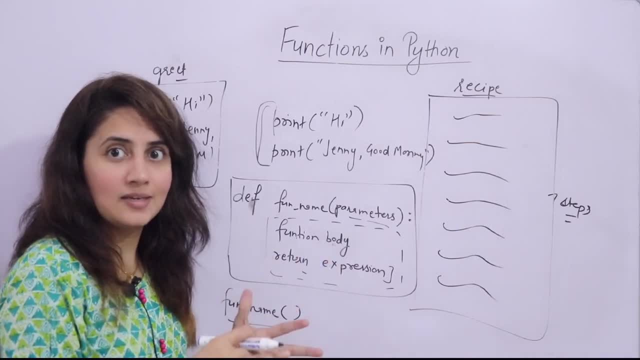 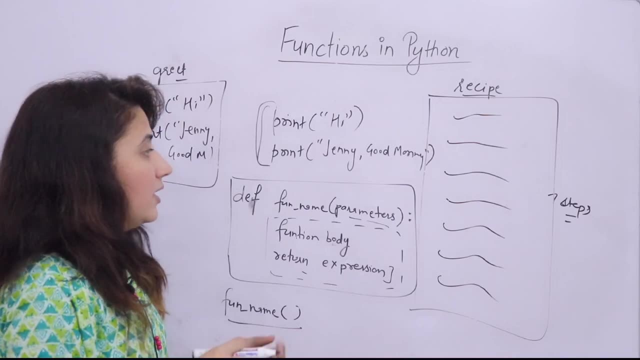 Means at that time students are calling me. You can say they are calling me. So at that time only I will work as a teacher, Right? So you have to call that function Right Now. there are two types of function: Built in function plus user defined function. So 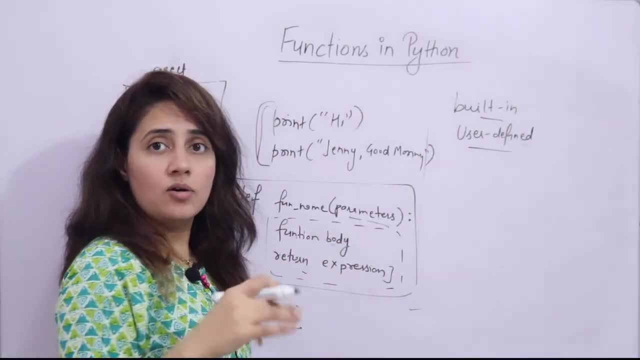 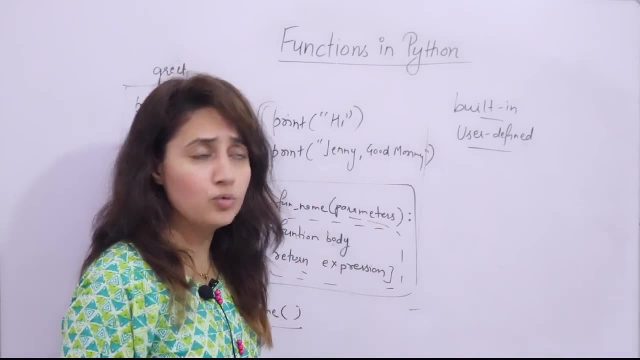 built in. functions are so built in. functions are already defined in Python, Already pre-coded or already defined. Right, You don't need to have need to write down any code to define those functions You can only use. you can directly use those functions Like simplest. 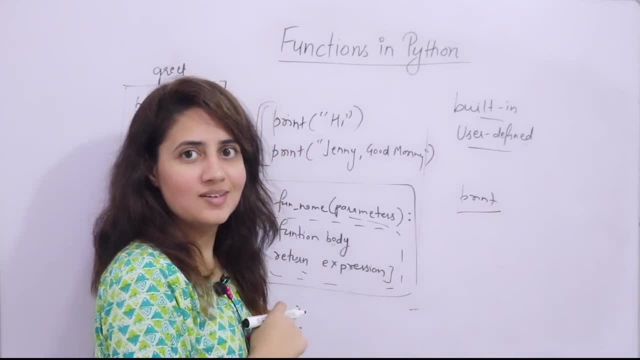 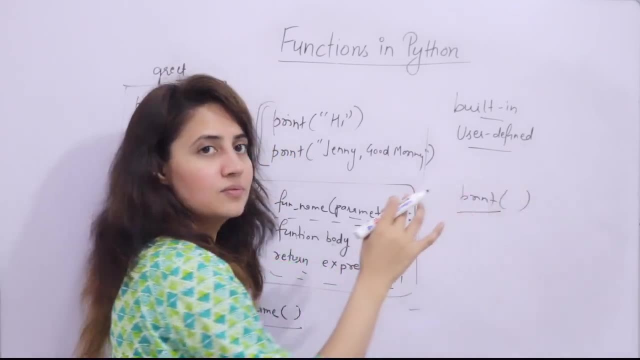 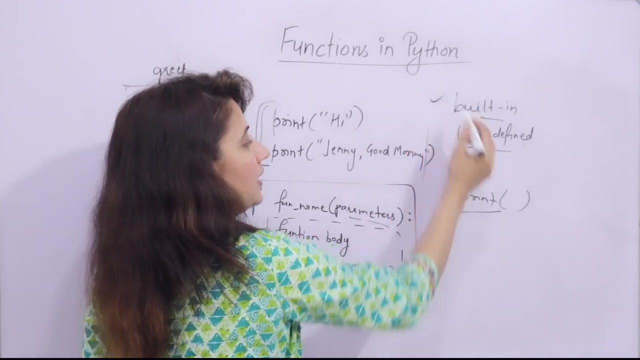 one is print. In every program we use this function. This is already defined in Python, So you just have to use that function. Just print in these parenthesis whatever you want to print that you can pass here. We pass that parameter, the argument Right Built in. 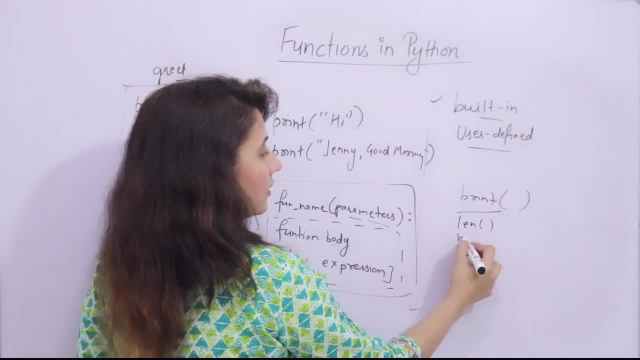 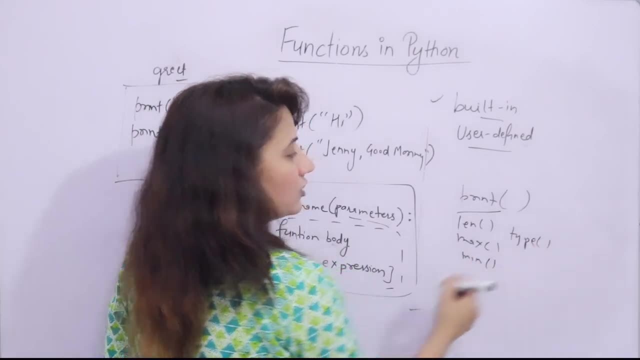 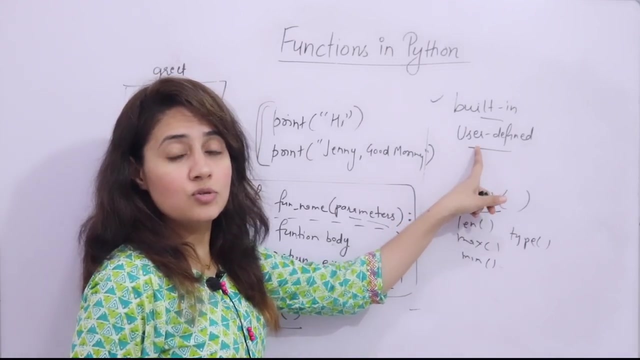 like print. we have len function. we have used This is also built in- Max, min and type also we have used Right. So many functions are there. You can also write down few built in function in comment section. Now next is user defined function. User defined means you have to define, user will define. 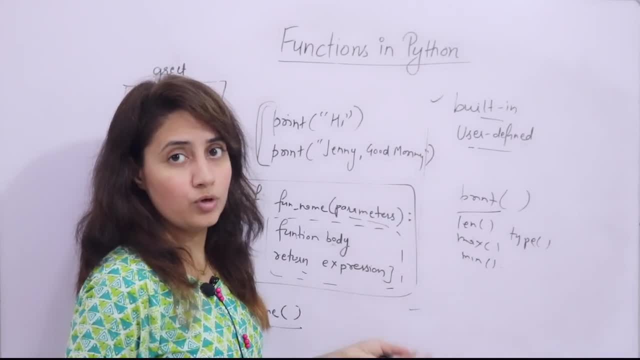 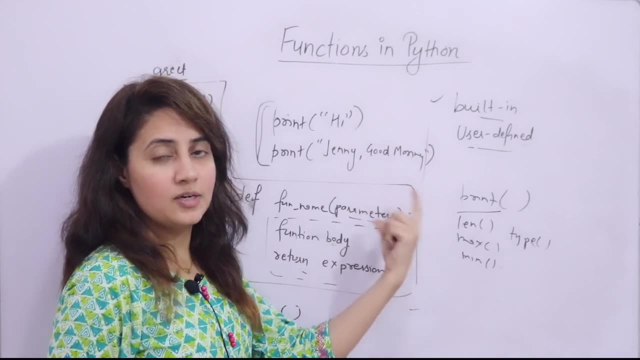 those functions as per our need, Like whatever you want. Like I want to define a function of addition of two number. So according to my need, I will define a function, The statement, the code I will write according to myself, Right, And how to define that I have told. 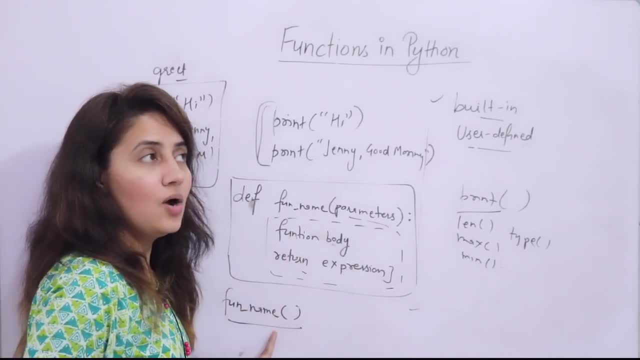 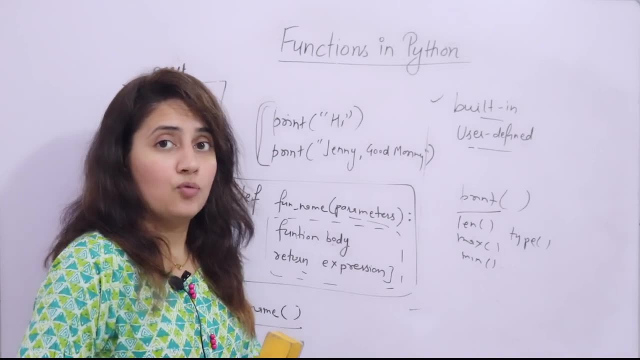 you How to call that. I have told you Right Now, let's see this thing with the help of example and I will introduce you with a new tool. So then you will get it better What function is and why we use it Now- the benefits or 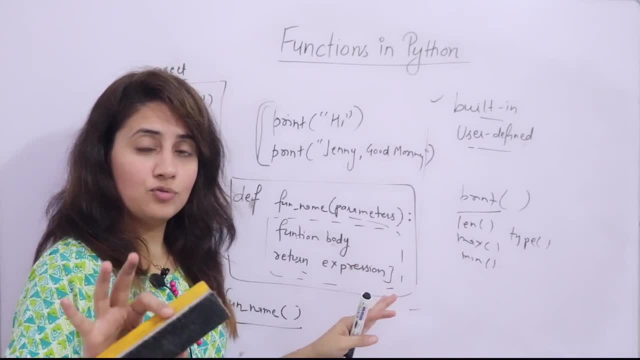 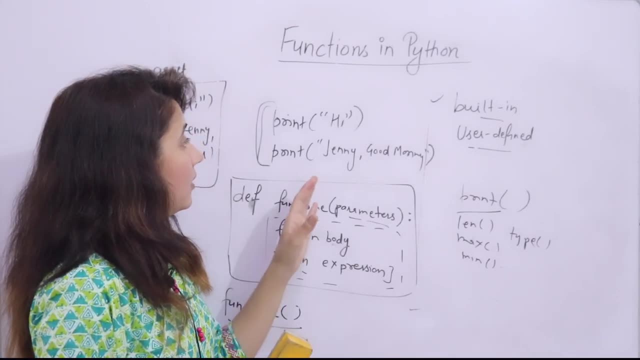 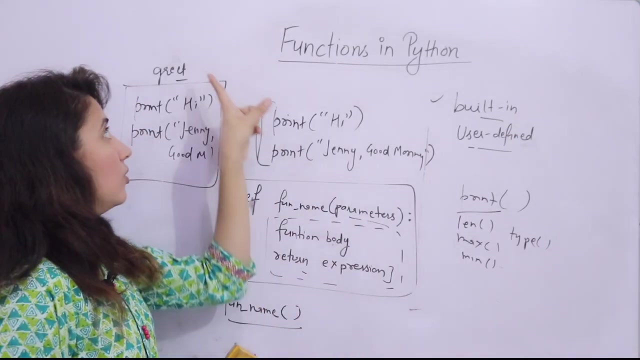 advantage of using function is what I guess. now you got it, What can be the benefits of using the function? Definitely, your code becomes more reusable. Rather than writing these two lines again and again in the program, just call the function. So means we are reusing. 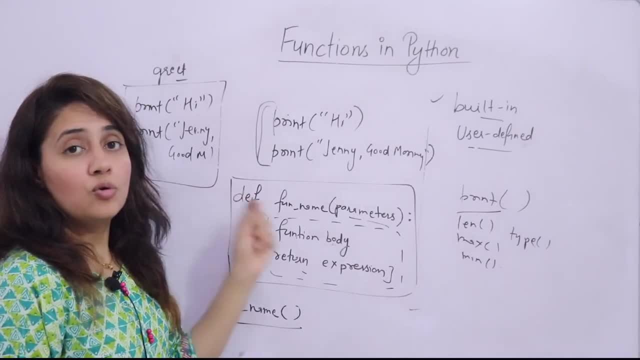 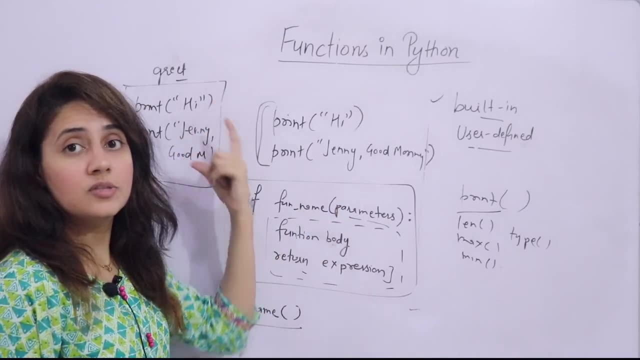 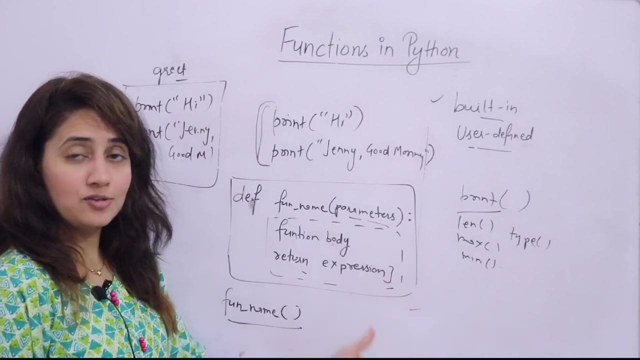 these two lines, So code reusability will increase. The code would be more readable, Right? Because obviously if you call a function, if you use functions, then the number of lines in your code will also is going to decrease, Will be less, And if less lines of code, then your code would be more, you can say, readable, Right. 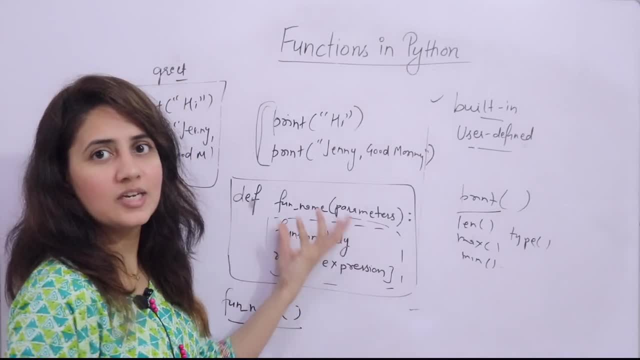 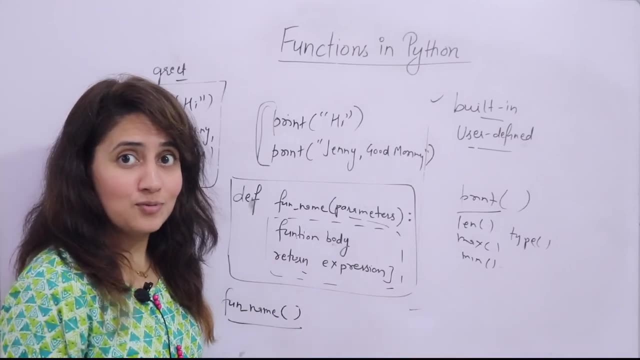 So these are few you can say and it will be time saving also, Right. Just define one time and use, reuse those thing again and again So it would be more readable Right Now. if time saving for you, right? Let me just show you this thing with the help of practical 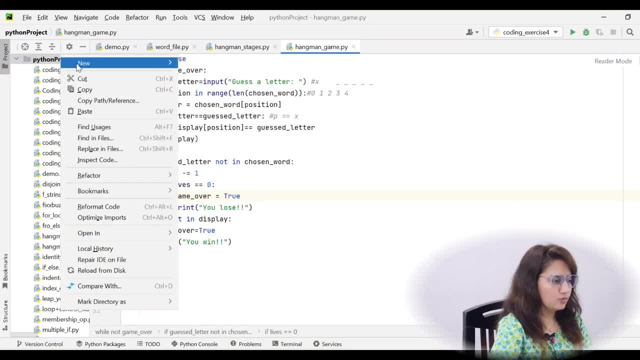 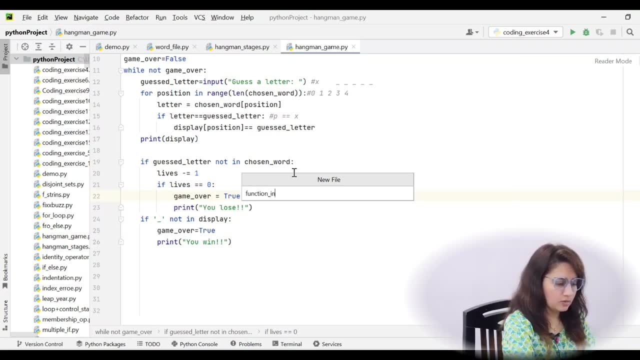 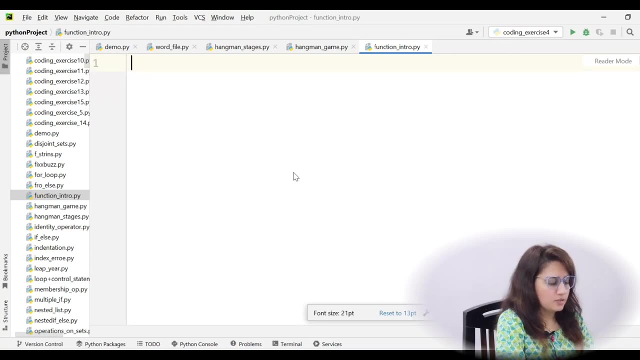 we will see a program on functions. ok, So let us create a new file here for functions, and functions like intro, dot, py, right, and let us define a function, def. how to define def? Let us take a function, suppose greet, right, colon, and here it should be indented. 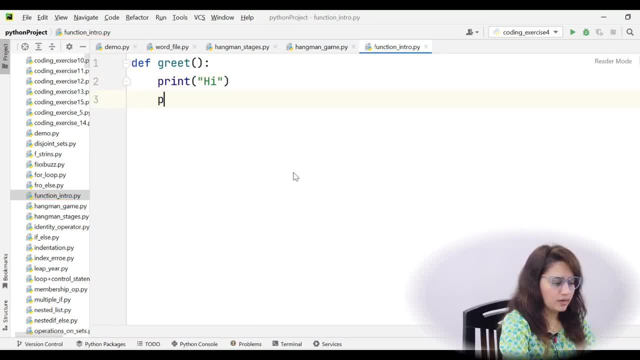 and there I just want to print hi in one line and suppose here I want to print only gen, these two lines. So now, this is definition of the function. we are not passing any parameter, because these are options. we are not returning anything here, right. So now, here what we. 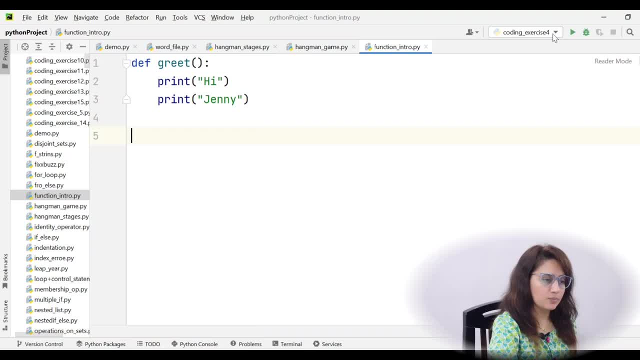 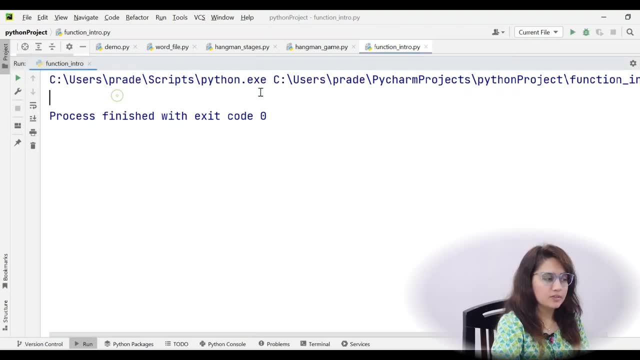 can do. How to execute the function. How to execute the function. How to execute the function. If I run this code, see, suppose we have defined a function. and let us run this code. see, it is not printing anything. the screen is blank, right? Why so? Because to execute the function. 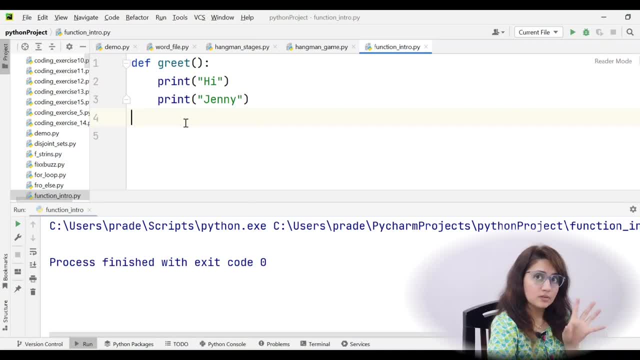 I have told you in the definition the function is a statement or block of statement, block of code perform, which performs some specific task when it is called. So you have to call the function, have to call the function. just name of the function: greet. that is it So. 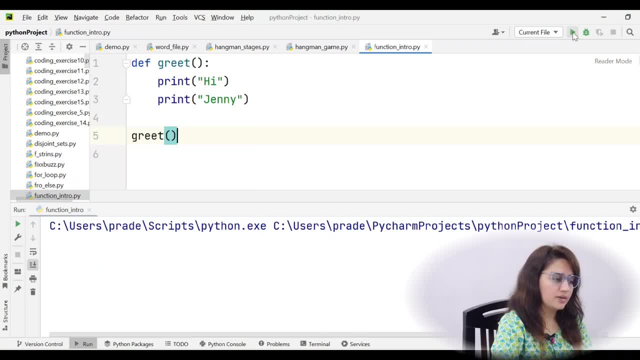 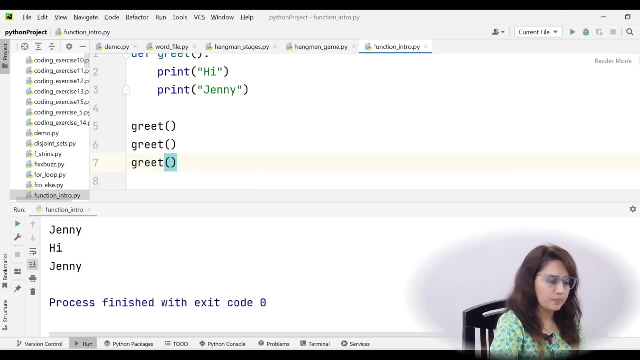 this is calling of function. Now let us run this, and this time it will print hi gen. So if you want to print this multiple time, so again I want to call greet again, like greet 3 times. So these two lines would be printed 3 times in your program. in the output see: 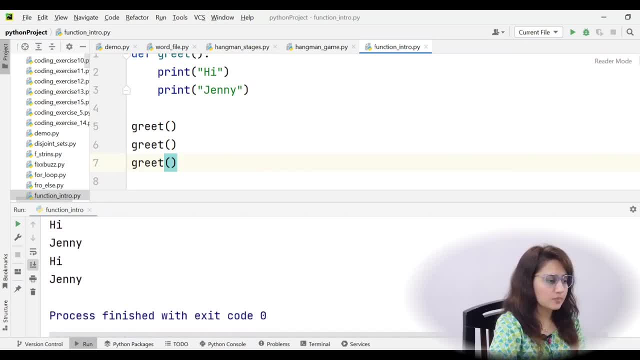 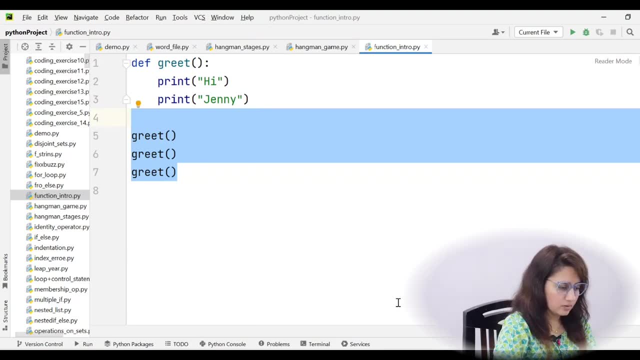 hi gen, hi gen, hi gen, right. so this is how the function will work. Now let me just introduce you with a new function. A new function is created, See, okay. So what I have done. So like tool we have rebox world. a website is there? okay, for that. you can directly search for like. 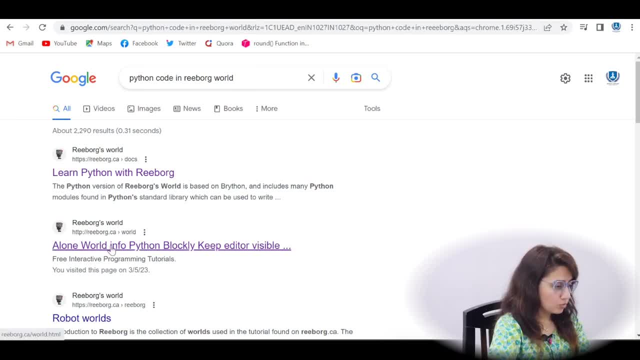 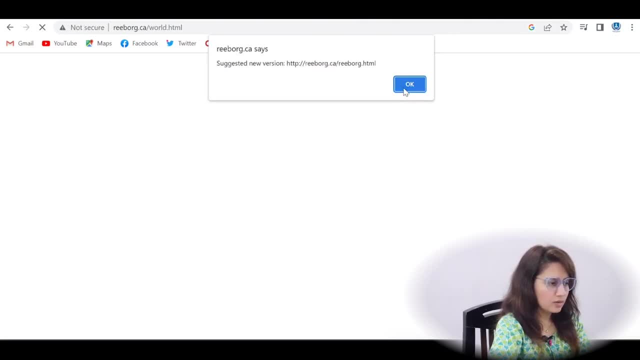 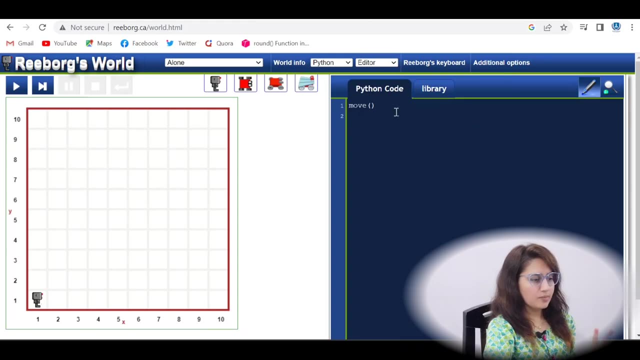 python code in rebox world. so first we'll take this example. this is the second link alone: world info python blocky. this keypad editor, visible right. let's run this and this is going to load right. so here this type of thing would be opened. here the project name is c alone, right. 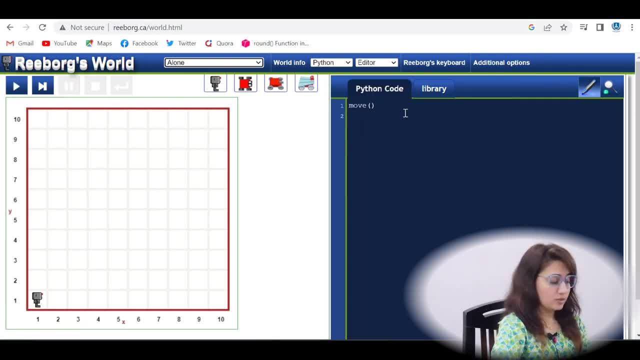 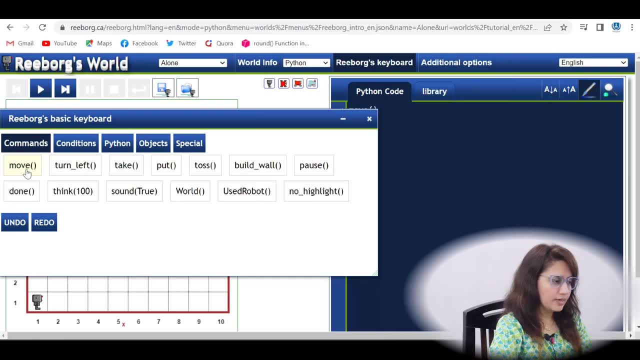 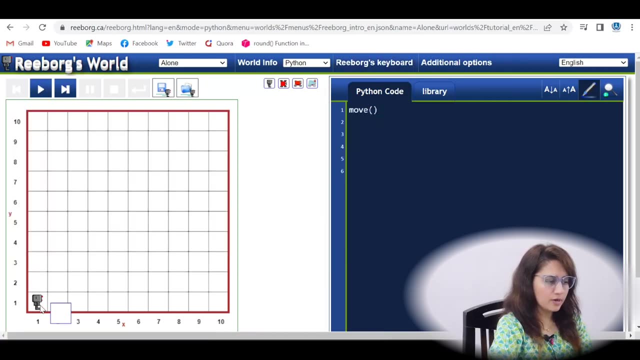 okay, now see the python code. here we can write on python code. so see, here we have some functions like when you click on this rebox keyboard, then you will get some function like you can say command, move, turn, left, take, put, these kind of commands. you can give these commands to this robot and 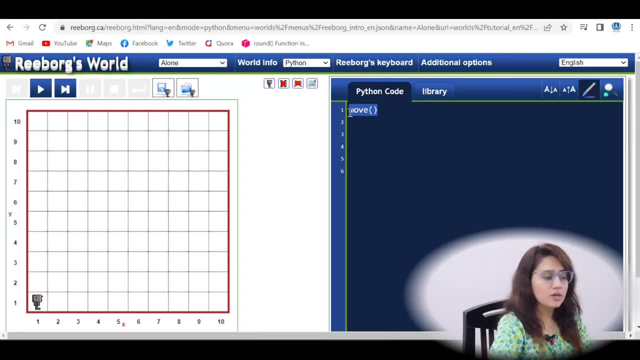 it will perform according to your given command. so here i have written one command like move. here we have one command: move. move means it will move further one step only. so how to run this? there's a play button right here. we have a play button right here. we have a play button right here we. 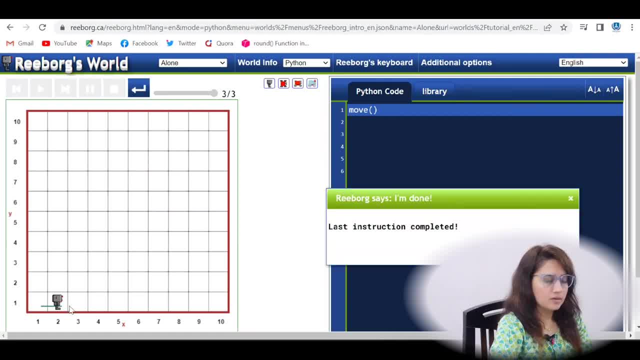 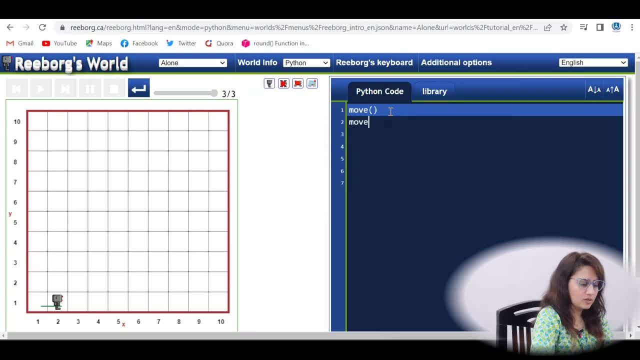 have a play button right here. just click on that and see it has moved one step ahead. so last instruction completed. so if you want to move this three steps or two steps, then just use this function again move or maybe three times move. and now, if you want to go back here, just click on this. 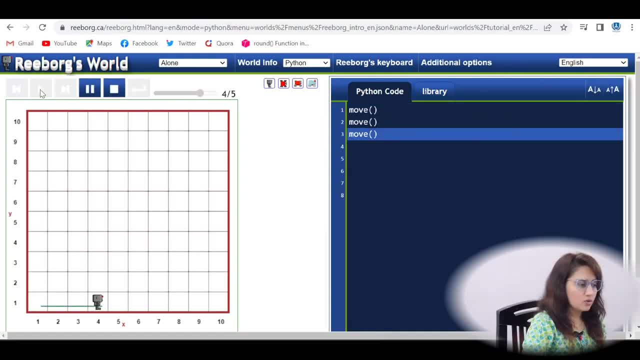 just go back this one and just click on the play so see it has moved three steps, the robot. so last instruction completed, right, so here we can write down our python code also. we haven't written till now. we are still you, we are using those. uh, you know, inbuilt function only we have. we haven't. 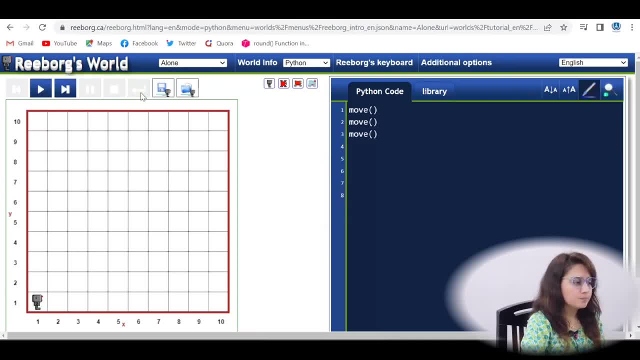 defined our own function till now, but we are going to define right now, if one by one, if you want to execute the instructions, suppose first instruction first and second and third, so you have to click on this one step through button, step click one, then see it is going to show this one line would be. 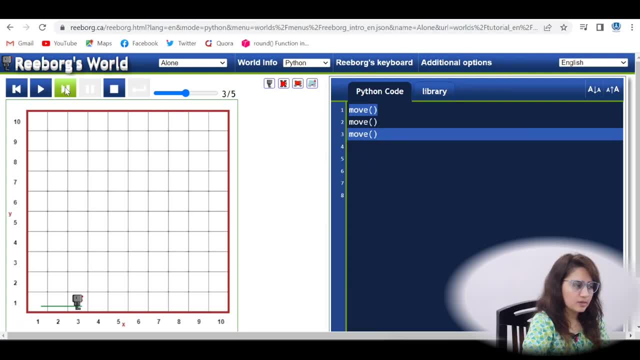 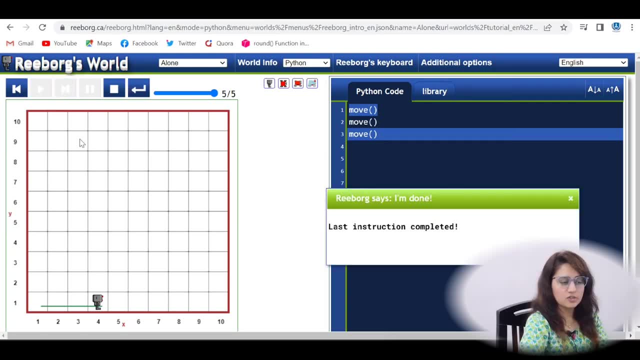 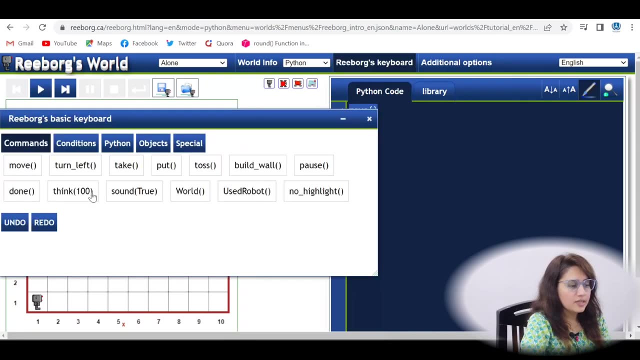 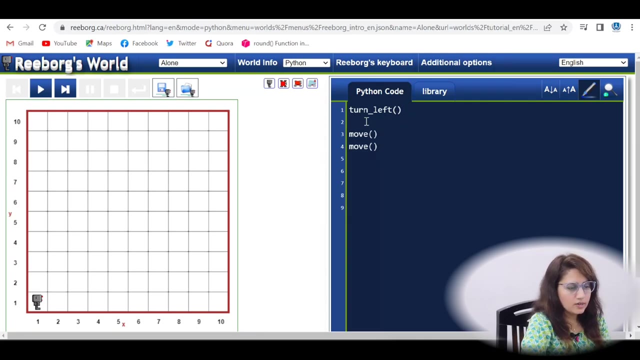 executed: move. see like this: again, move, again, click, move, three line would be executed and that's it, last instruction completed. so let's back here and, okay, turn left. there is one function, use this turn left. just click on that and it would be here: turn left, or rather than first, turn left, first we move. 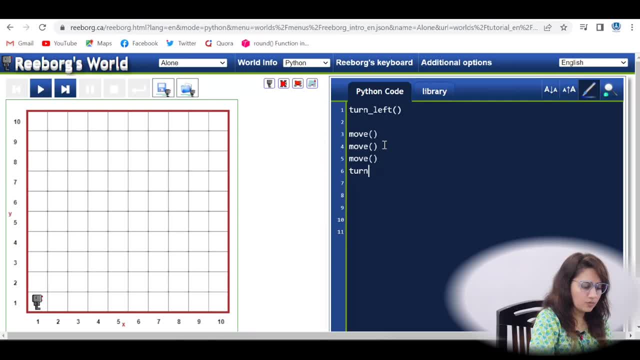 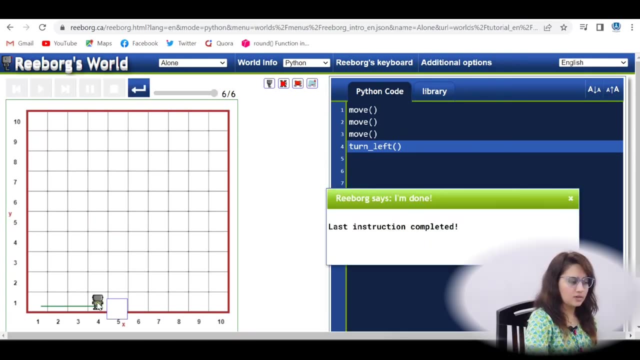 this robot like three times and then we use the function turn left, not at the starting. so if i run this code here, so three step. then turn left, see, turn left. the robot has turned left this way it is going. then turn left this side and again, if i 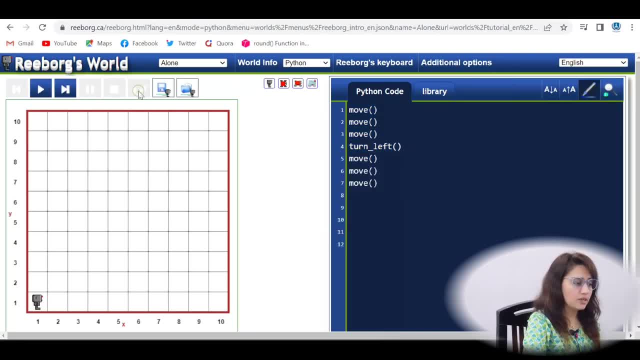 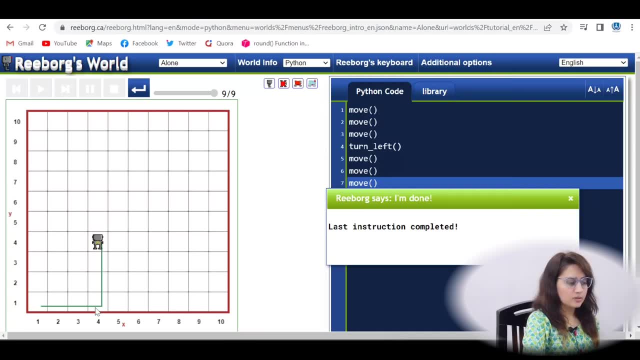 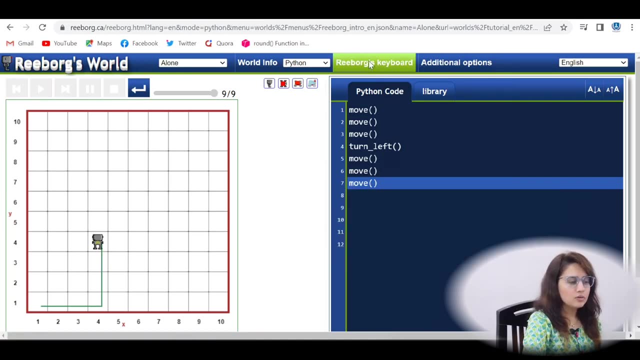 after turn left, if i use the move function again three times and if i run this again, see now this would be executed: move first three times, turn left and move again three times right. but there is no, see, there is no turn around or turn right function here. right, only turn left is. 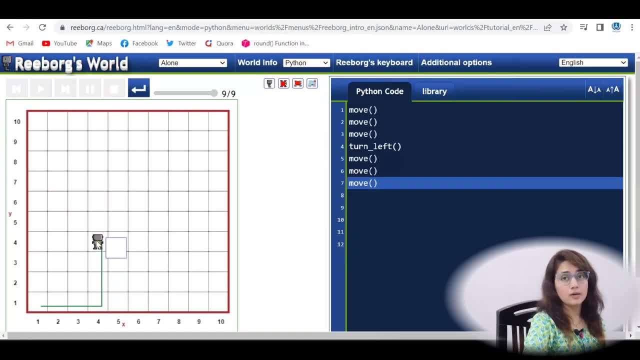 there now. if you want to here command the robot to turn right, then how you will give that thing? so define your own function: turn right function at this point of time. if i want to give the command to this robot turn right, then how will you now? you have to define your own function now pause. 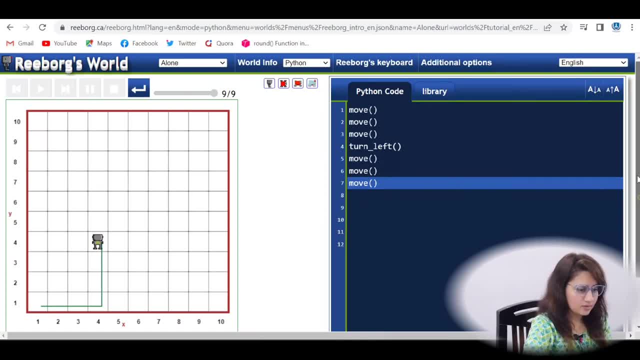 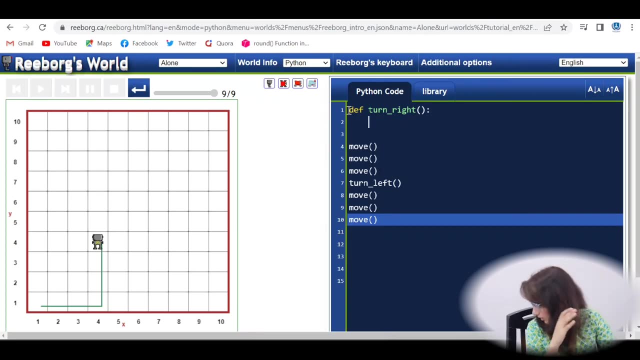 the video and define your own function. okay, how you are going to define def keyword function name. i am taking turn right, parenthesis, colon and now the definition. it should be indentation right now. turn right means simply, at this point of time, if this robot, we give this robot three times turn left command, then it would be automatically at the last. 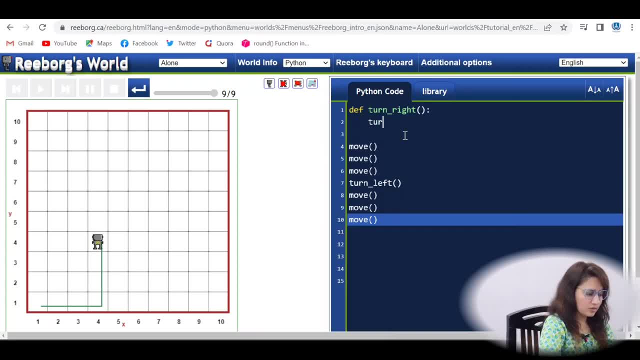 ultimately turn right command would be executed. so three times turn left. so now this is a turn right function. now, now, if i call that this function here, turn right, and suppose again move, one step move, and if i run this, let me just stop this, just click on this. 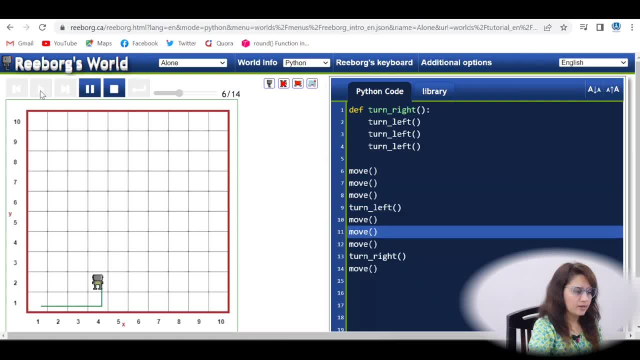 reload button and play like this: right, turn, right and then one move. but we have defined our own function, suppose, if you want to execute this, if you want to command the command, this head and side button, this, you know robot, something like this. okay, the same thing then. 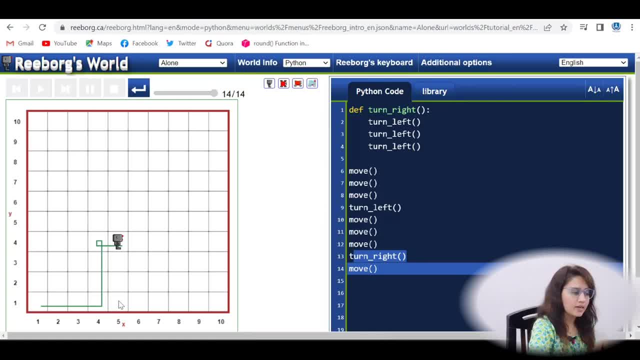 it has to move downward, three step right again, and then simply the face would be in this, in this direction, only this direction, forward direction, only right. so how you are going to give this, this, this command. see now, at this point of time, also for going downward you have to give the command obviously, turn right. like this we are facing. 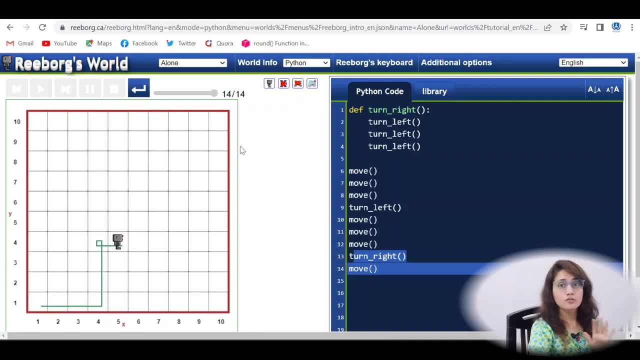 then at this point of time means turn right, right. And if suppose you haven't defined this function, then for turn right you have to write down this turn left 3 times. So here, rather than turn right, you have to write down these 3 times, Then again, move, then again. 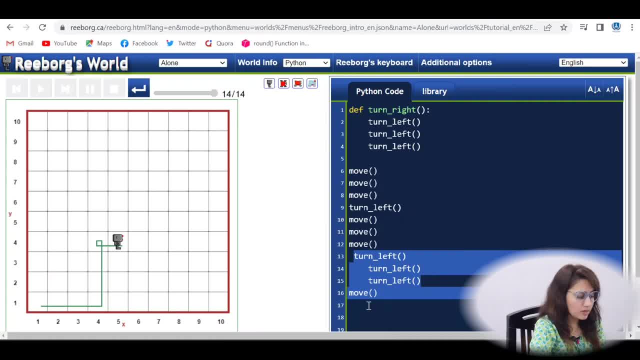 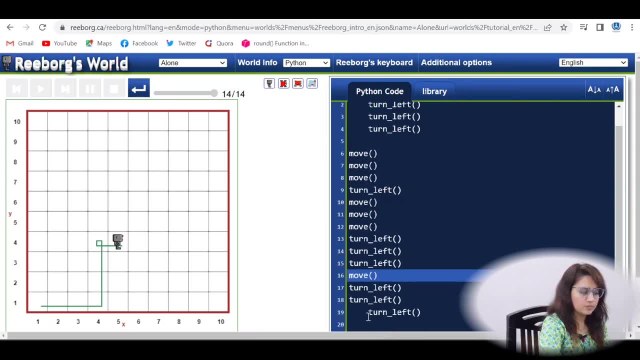 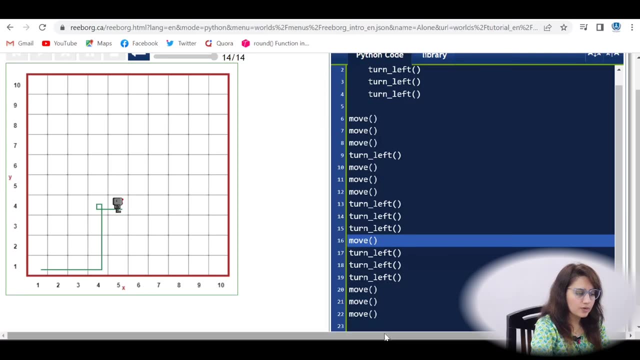 turn right. So again write down these 3 commands: turn left command here like 3 times. Here there should be no indentation right Now 3 times. move right And then finally turn left right. This would be the case if we. 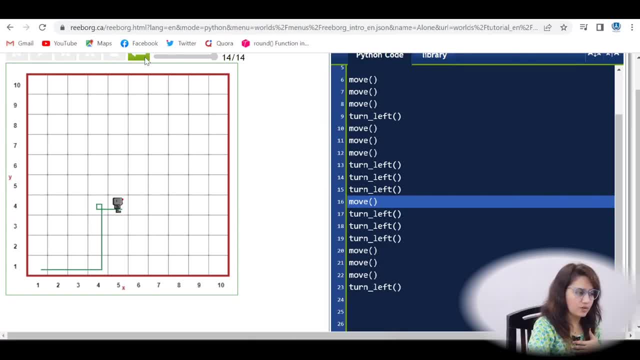 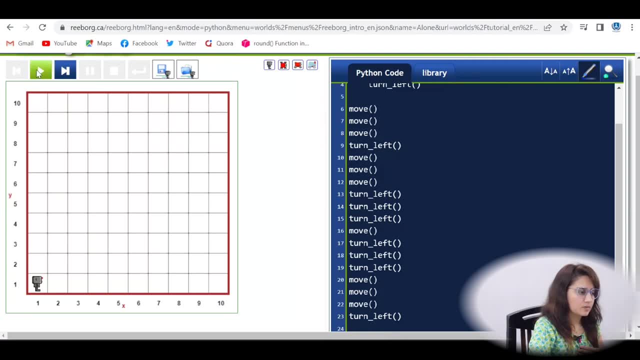 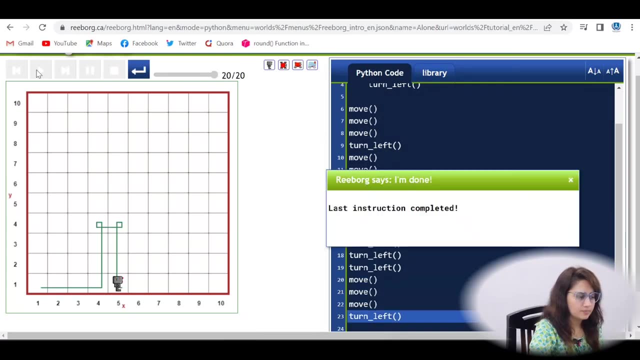 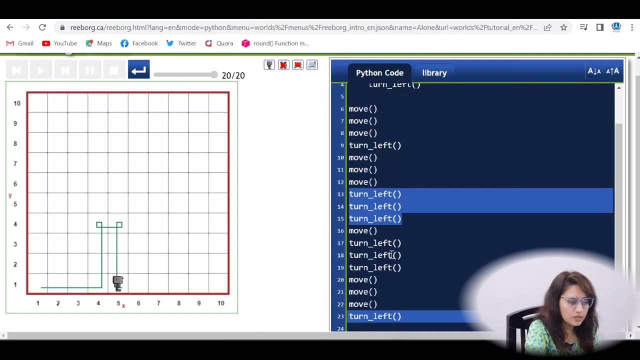 are not using the function turn right, we haven't defined the function, So let's stop this. and now let's run this. Yeah, leave it, go, Here we go. So now you are repeating these turn left and turn left, these 3 lines again and again. Whenever you want to give the command to the robot turn. 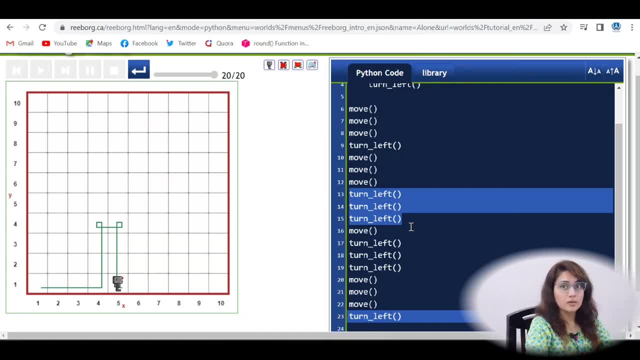 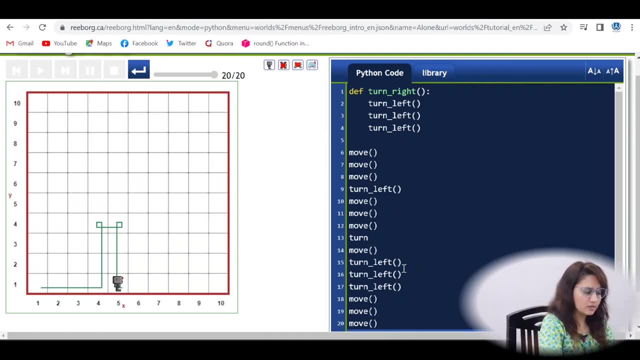 right, then 3 times you have to write down turn left again and again. So better to define a function. So that's exactly we have done: just define a function, turn right, and rather than these 3 lines, just use one line: turn right, that's. 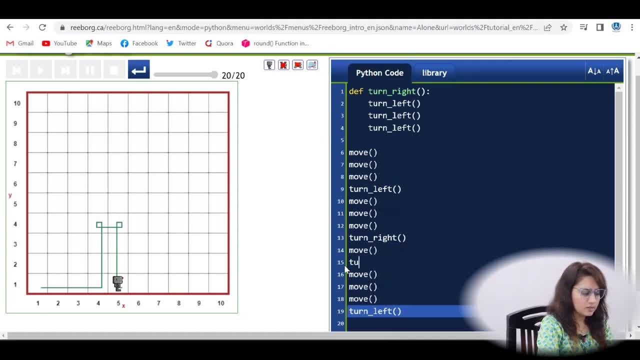 it, rather than these three lines. just type a solution- right川ально operation- and ask the debate. Erm like, just give those 3 lines. 3 lines, bang, bang, bang. just start now turn right, just one line. So yeah, this is going to reduce the number of lines in. 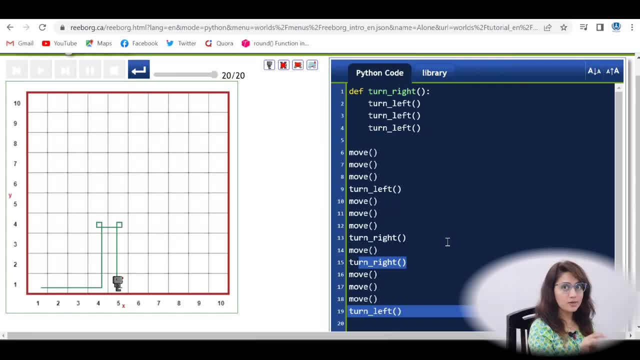 your code When you are using function. code reusability will increase and as well as code readability will also increase. right, This is also going to perform the same task One by one. we are going to run this now, this step through option. Let's run this Once. 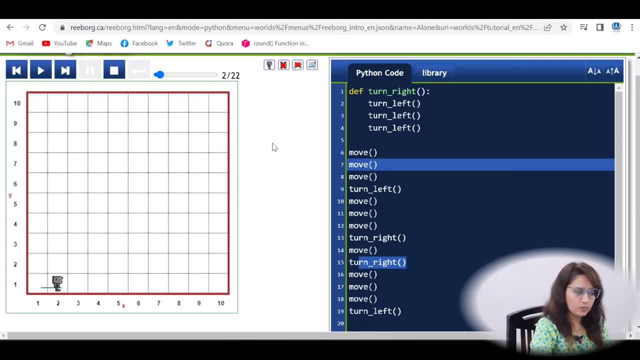 click, then again click, Then this move command will be executed. Then second move: Again. run again. turn left again, again again. click on that Now. see cursor is here at this function. turn right Now. click on the step function. Now cursor would be here in. 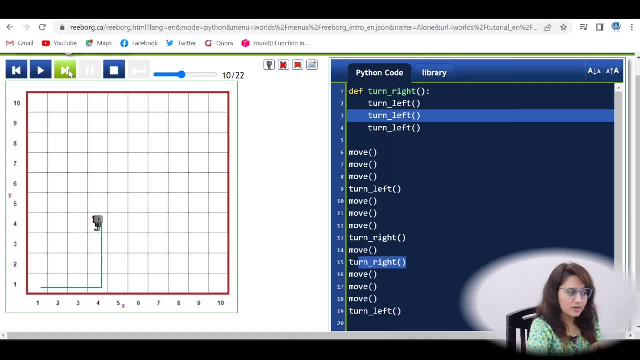 the definition of this function. So first turn left again, second turn left, again, third turn left Would be performed. now, That's it, Now we are, we are turning, we have turned right this robot, Then move, then again turn right, then again function would be called See. 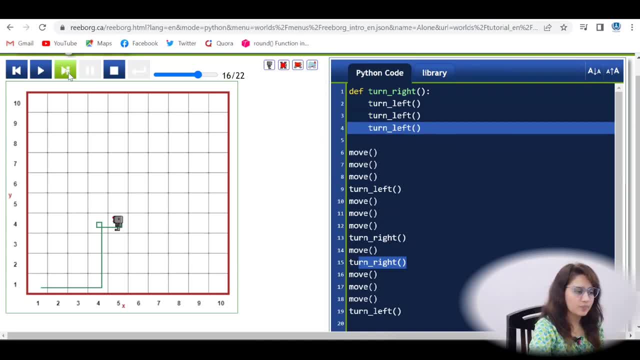 the cursor is again, the control is again here within the function. Then three times turn left and then move, Then this move, then this, then again turn left and that's it right. So this is beauty of function you can use. 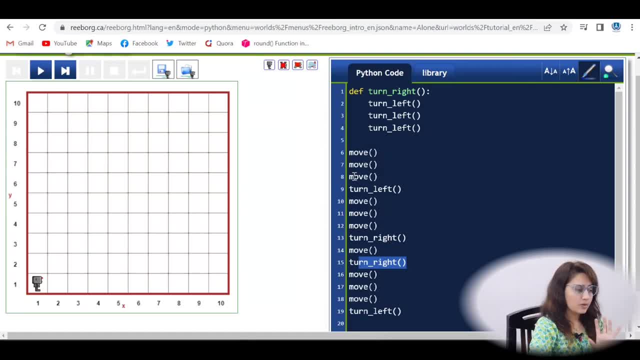 Now one exercise for you is turn around. There is no function turn around here, So you have to define your own function, how to turn around. Let's suppose move this robot three times here, three times forward, then turn around, then three times backward. the 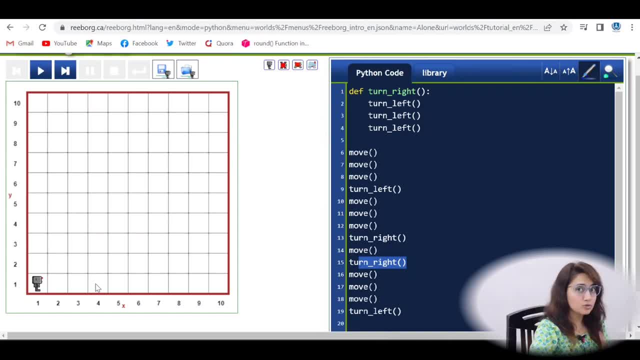 same position How you will define your turnaround function. Pause the video and try this out. Okay, Okay, Okay, Okay, Okay. I hope you have done this. how to define turn. I think this is very simple If you have done this. turn left and around is very simple: Just two times turn left and that's.